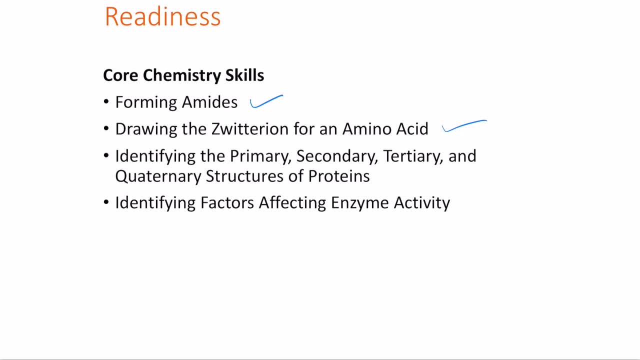 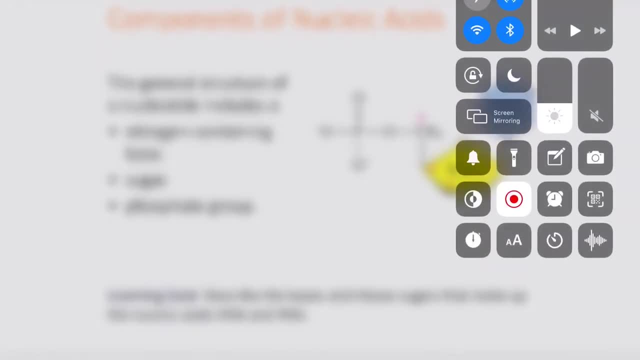 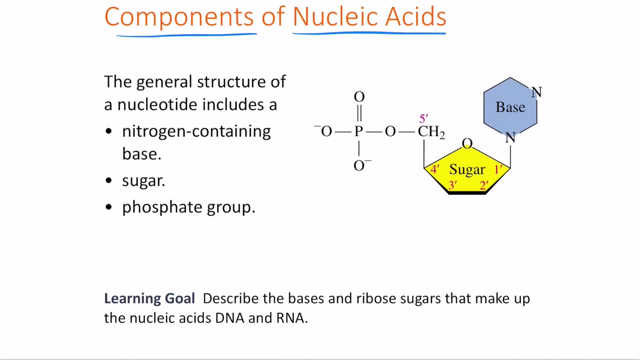 drawing the zetarion of an amino acid, identifying the primary, secondary and tertiary and quaternary structures of the protein and identifying the factors that affect enzyme activity. So now let us start with the components of nucleic acids. So the general structure of a nucleotide includes three things. One: you have a base. 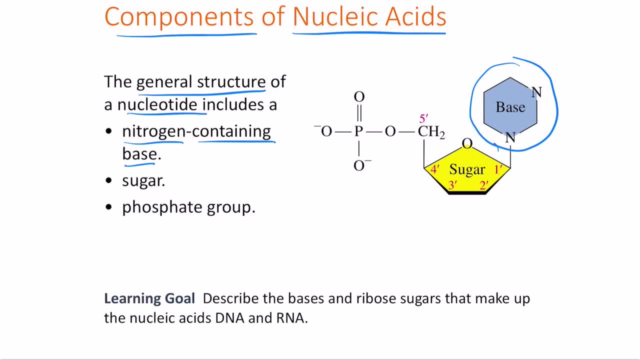 which is a nitrogen containing base, You have a sugar and you have a phosphate. So these are the three main things that you need to understand the idea of a nucleotide. So whenever you see the term nucleotide, so remember that there are three things that are involved. 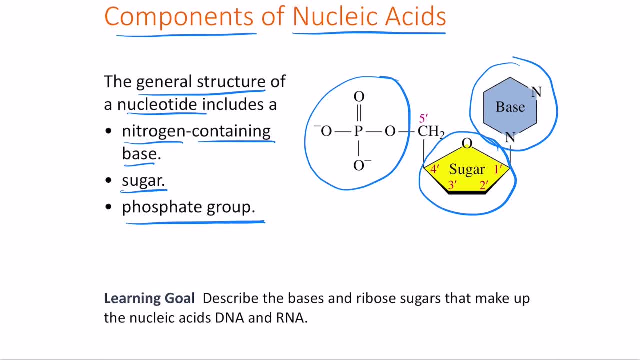 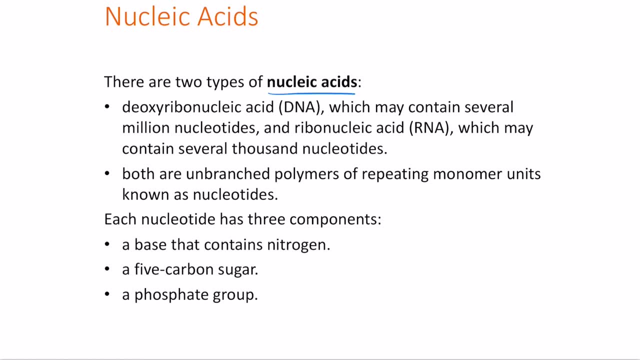 So there are two types of nucleic acids. The one is deoxyribonucleic acid, and which may contain several million nucleotides, and you have ribonucleic acid, which may contain several thousand nucleotides. So, in general, remember that DNA is longer than RNA. So 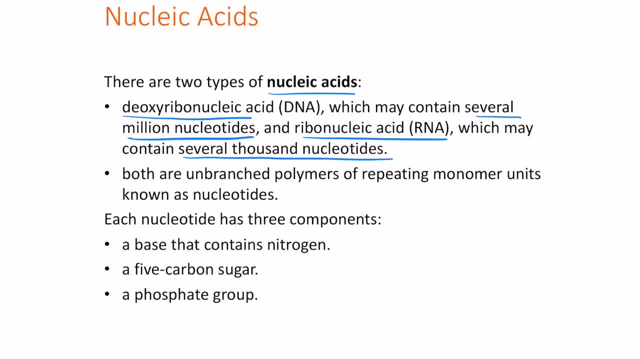 DNA is larger and much more complex structure than RNA, So both of these are unbranched polymers of repeating monomer units. We call them nucleotides, So think of them as nucleic acids are basically unbranched polymers of nucleotides, So each nucleotide contains: 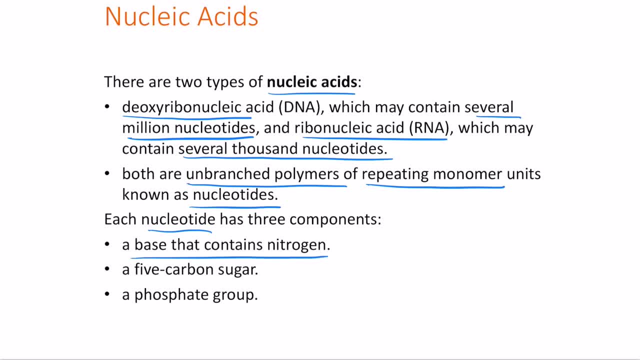 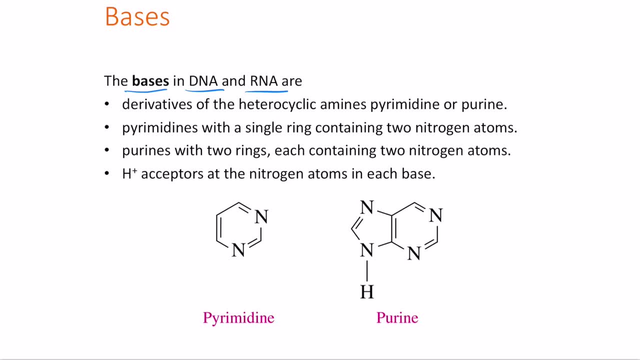 three things. So one: you have a base that contains nitrogen, a five carbon sugar and a phosphate. So the bases in DNA and RNA are generally derivatives of the heterocyclic amines. So the heterocyclic amines that are involved are two of them: One is pyrimidine and purine. 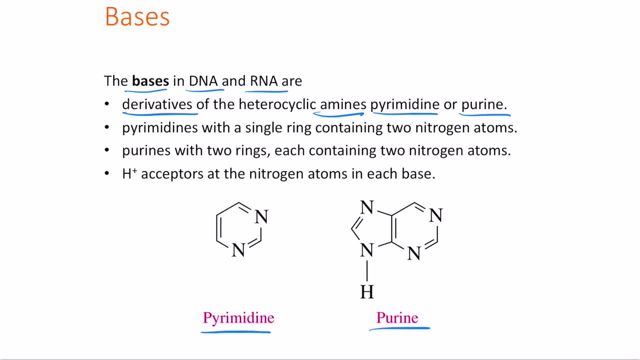 So these are the two bases that are involved. So pyrimidine is a single ring containing two nitrogen atoms. Purine contains two rings: One is a pentagonal ring, the other is a hexagonal ring, combined in a bicyclic structure, each of it containing two nitrogens each. So there, 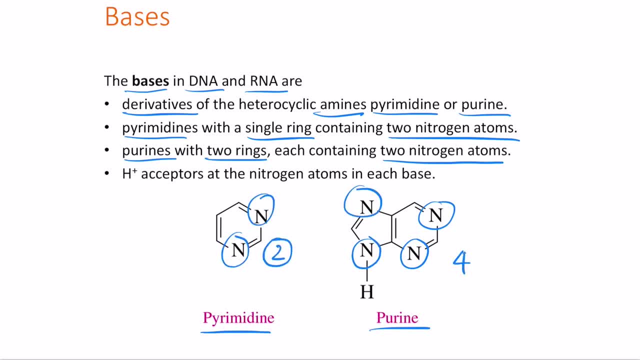 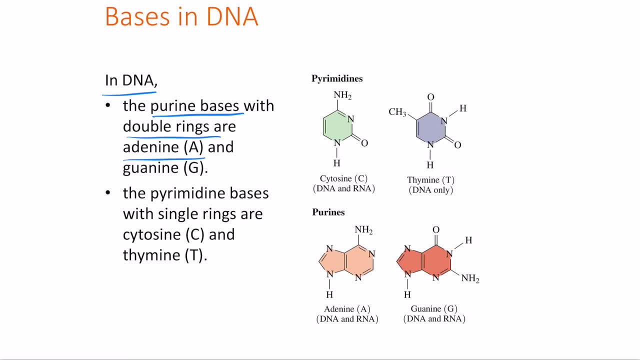 are four nitrogens here and two nitrogens in pyrimidine and four nitrogens in purine. So in DNA the purines here with double rings adenine, and they are called adenine and guanine. So there are two pyrimidines in your structure. One, you see, is DNA and the one is cytosine. 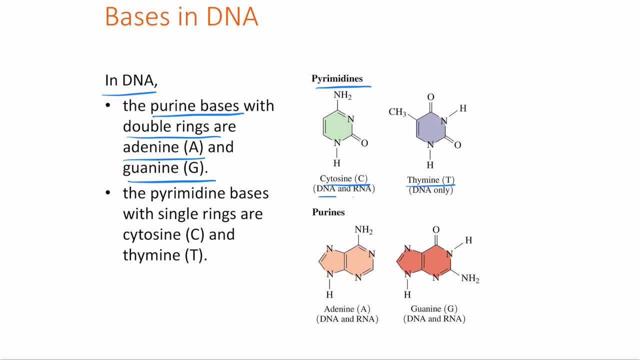 and the other is thymine. So cytosine is present both in DNA and RNA. Thymine is only present in DNA. So the pyrimidine bases with single ring, with single rings, are cytosine and thymine. You have purines, purines that are adenine and thymine. So these are the 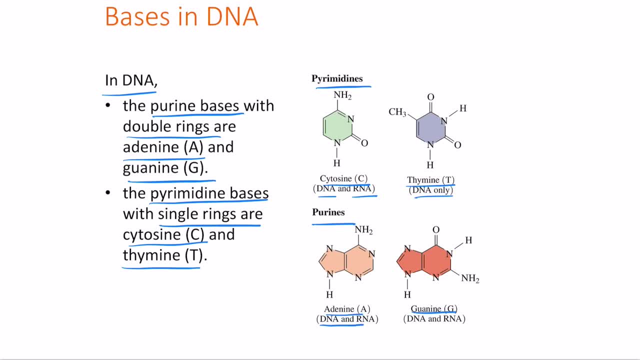 main bases. So the permutations are adenine and guanine. Adenine is present in both DNA and RNA. Also, guanine is present in both DNA and RNA. So in RNA you have two rings, Again the purine basis. the double rings are adenine and guanine, So the pyrimidine. 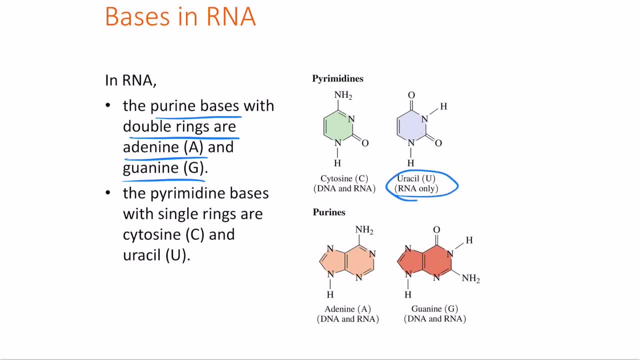 bases that you find only in RNA is the uracil. So in DNA you find four of them, So we give them the shortcut C, T for pyrimidines and A G for pyrimidines. So in DNA you find four of them, So we give them the shortcut. 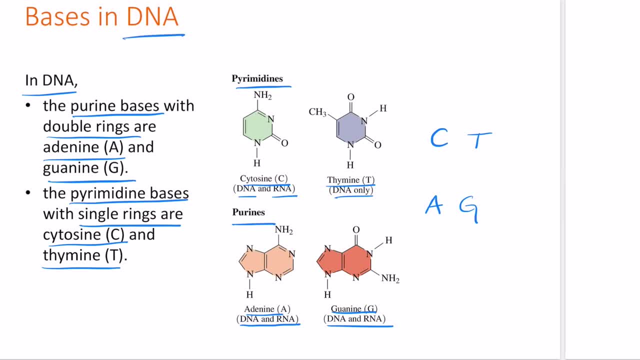 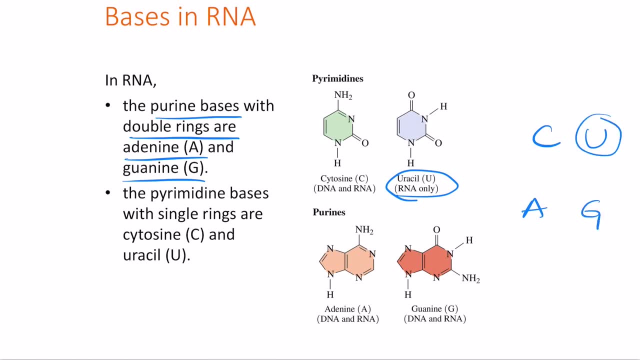 purines. so this is the ones that are present in dna only, and in rna you get c, u a, g. so in place of thymine you get uracil. so the only difference in structure is the presence of a methyl group, so his presence of a methyl group. so if that methyl group is not present, it becomes uracil. 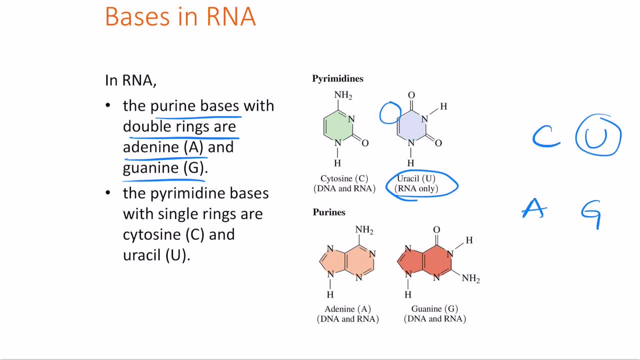 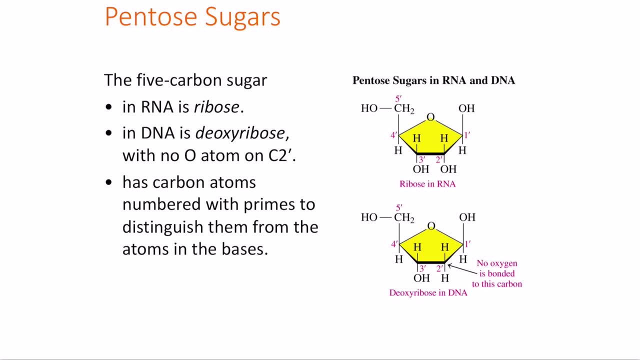 if that methyl group is present, it becomes thymine. so this is the difference here between the bases that you are that represent in rna and dna. that is the main structure that differentiates a rna and dna, and the second thing that that can separate a dna and an rna is the sugar itself. the 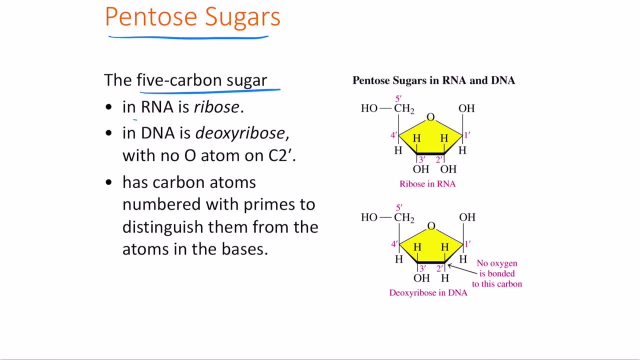 pentose sugars, so the five carbon sugar in rna. here is a ribose. so ribose involves: you have oh groups on all of the carbons except for the sorry. you have oh groups on all of the carbons except for the fourth carbon. but the difference in a deoxyribonucleic acid is in this second. 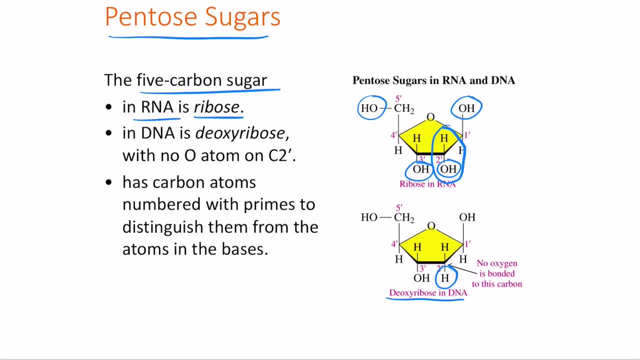 carbon. so there is no oh group present in the second carbon. here both of them are h and h. that's the reason why the term deoxy ribose. so remember that this is basically a ribose without the oxygen. so we are saying that we call it a deoxyribonucleic acid with no oxygen. 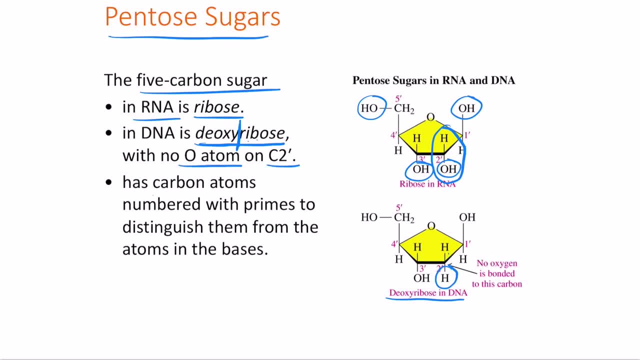 atom at the second carbon, so the five carbon. sugar also has carbon atoms that are numbered with primes To distinguish them from the atoms in the bases. So remember that the atoms are different and the carbons are different, So the carbons are named separately. So we always name the prime structure and prime. 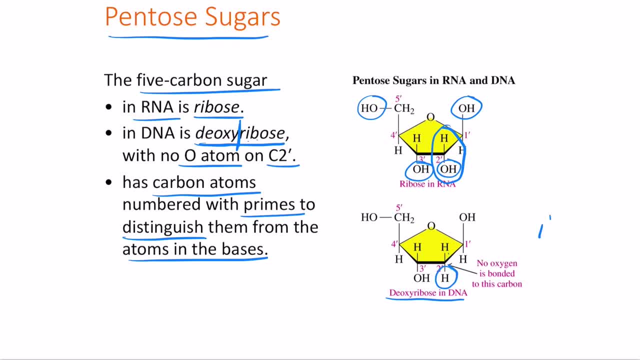 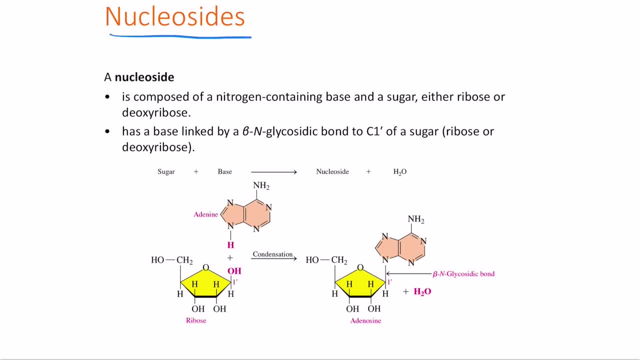 numbering for the. we just put one prime, two prime for the carbons to differentiate it from the other other atoms. Next, the other type of an atom is called as a nucleoside. A nucleoside is basically a composed of a nitrogen containing base and a sugar. Remember that the nucleoside plus a 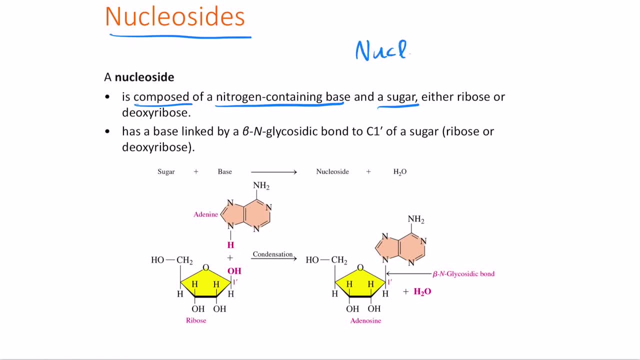 phosphate group is equal to the nucleotide, So a nucleoside is a nitrogen containing base plus a sugar Right. So this has a beta nitrogen glycosidic bond. So it generally bonds with the H and OH bond here and go out, resulting the addition of the nitrogen and the hydrogen. 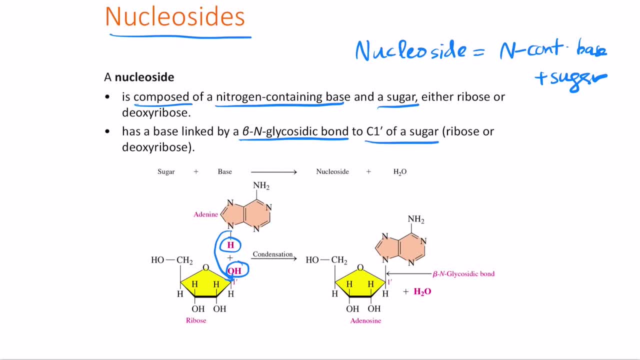 So this bonding occurs here, and this carbon one bond results in the addition of the hydrogen and the hydrogen. So this bonding occurs here, and this carbon one bond results in either a ribose or a deoxyribose. It can happen with both a ribose and a. 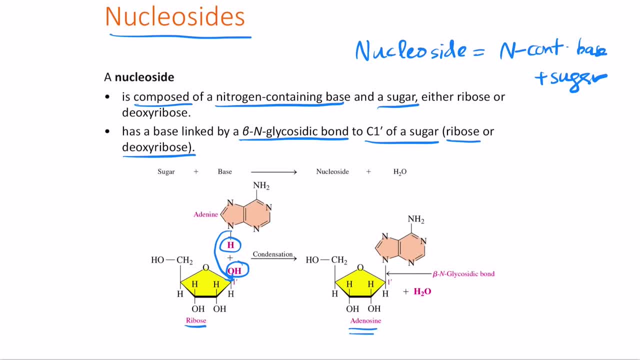 deoxyribose. So the most common acid, most common sugar that it bonds with is adenosine, So we call it adenosine nucleoside. So a sugar and a base combine to form a nucleoside and H2O. Next comes. 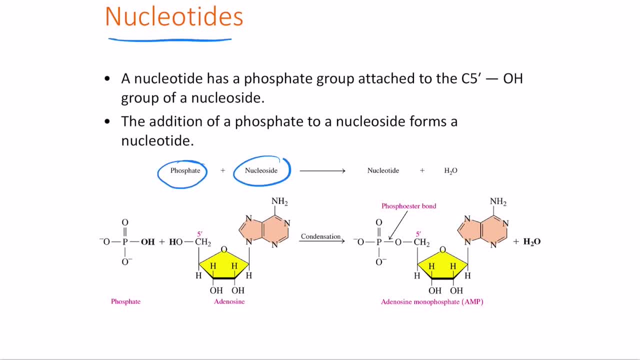 nucleotide. Nucleotide is a combination of a phosphate and a nucleoside. So for a nucleotide to form, you need a nucleotide and a nucleoside. So for a nucleotide to form, you need a nucleotide and a nucleoside plus a phosphate. So a nucleotide here has a phosphate group. that is attached to. 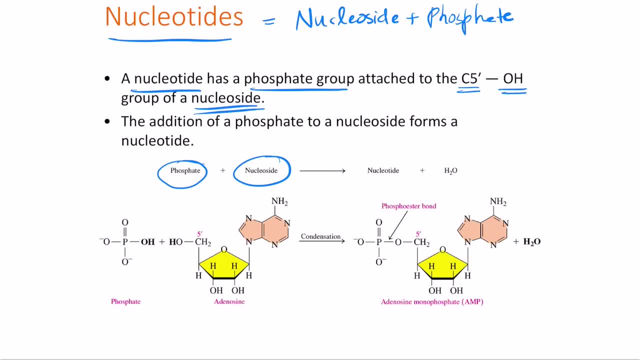 the fifth carbon on the OH group of the nucleoside. So here, remember that the nitrogen base attaches itself to the first carbon and the phosphate attaches itself to the fifth carbon. So the one and five are the main important bonds that you have to remember. So for the first carbon, 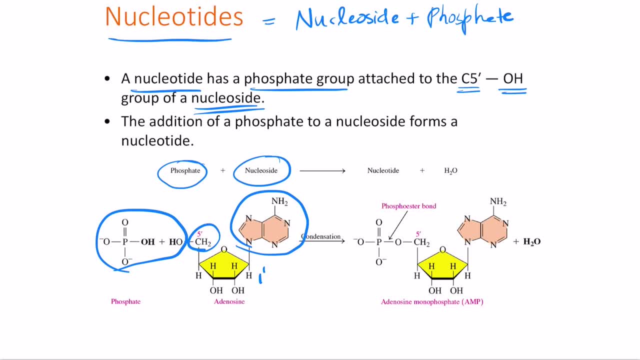 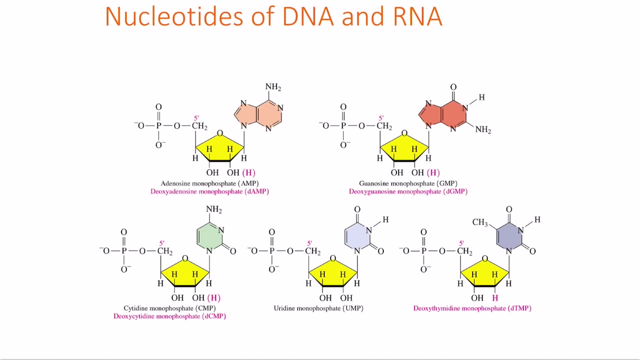 it involves the bonding with the nitrogen base and the fifth carbon involves the bonding with the phosphate base. So when phosphate and nucleoside involve, it creates a nucleotide and it releases water. So there are there are in total five types of nucleotides in total in both of RNA. 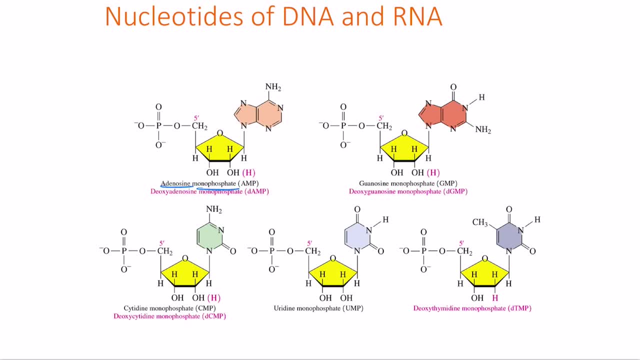 and DNA. First one is adenosine monophosphate, So this is AMP, where the sugar is adenosine. Sorry, the base, the nitrogen base, is adenosine adenine and you have guanosine monophosphate, So where you have guanine. 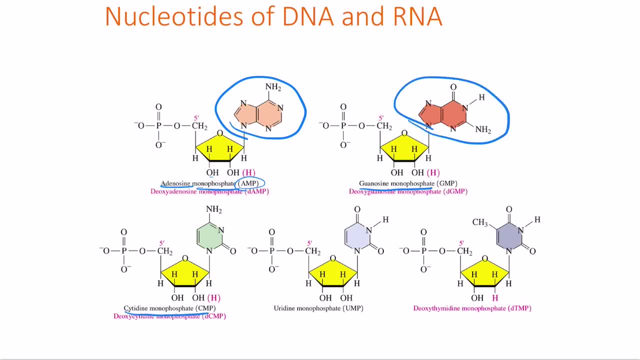 is the nitrogen base. You have cytidine monophosphate, which means cytosine- here is the nitrogen base. You have uridine monophosphate, which is, which means uracil, is the nitrogen base, and deoxythymidine monophosphate, which is going to be resulting in the formation of a thymine. 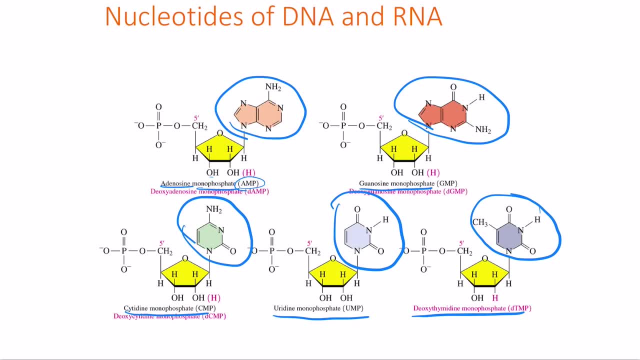 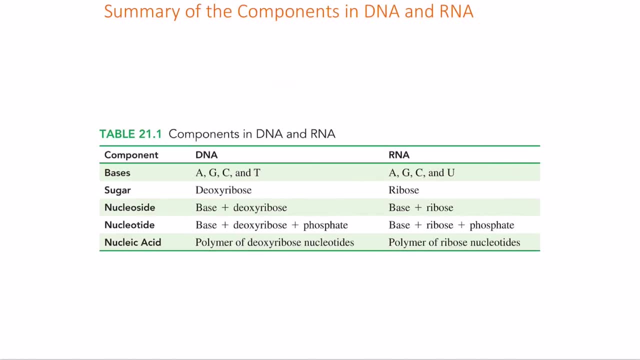 base. So these are the five bases and out of them, this is only present in RNA, It's not present in DNA. So the components in DNA, you get AGCT as the base. In RNA it is AGCU and the sugar here is a deoxyribose sugar. 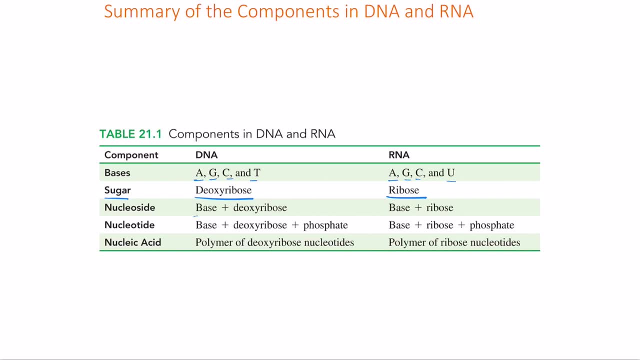 Here it's a ribose sugar. The nucleoside involves the addition of a base and a deoxyribose. In RNA it involves the base and the ribose, And in a nucleotide it involves base plus deoxyribose plus phosphate. In RNA it involves base plus ribose. 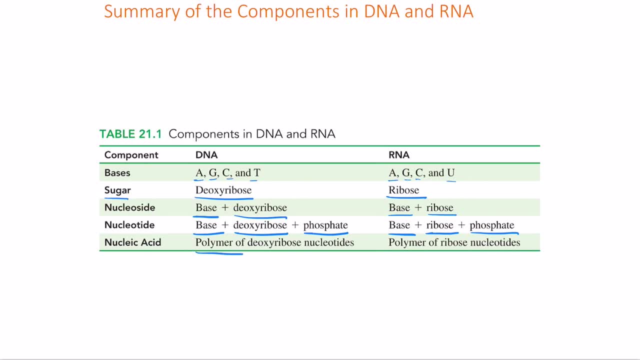 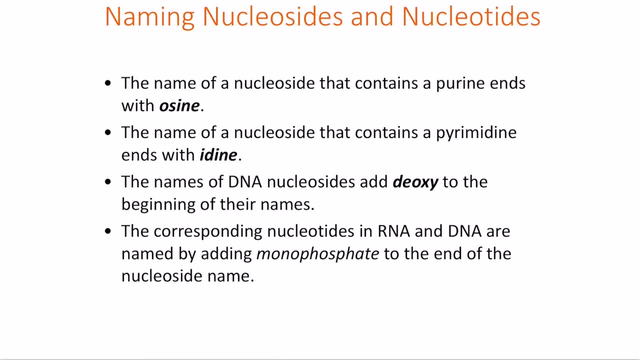 And the nucleic acid is a polymer of deoxyribonucleotides, and RNA is a polymer of ribonucleotides. Now, so the name of the nucleoside generally ends with contains a purine, that ends with osine, and the name of a nucleoside that contains a 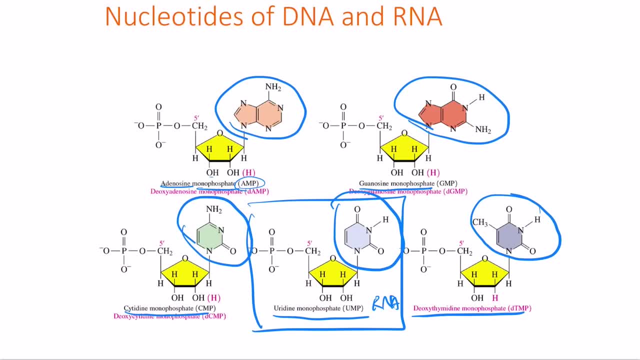 pyrimidine generally ends with edine. So that's the reason why notice that it is adenosine, because it is a pyrimidine, So it's a purine, and you have guanosine, which is again a purine. So remember that. here the idea. 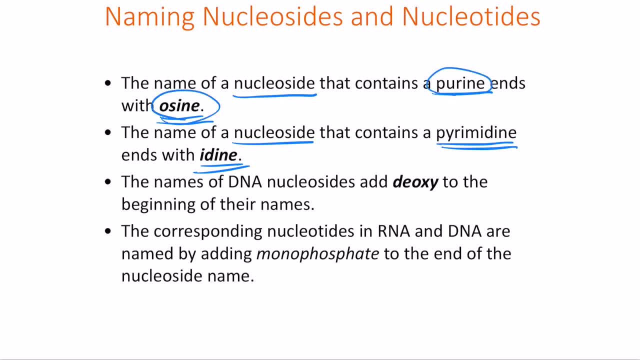 here is that if it involves a purine, it becomes, ends with osine. If it's a pyrimidine, it ends with edine. So this is how we can differentiate with what type of base it is, whether it's a purine or a pyrimidine. Now the name of the DNA nucleosides add deoxy to the beginning of the. 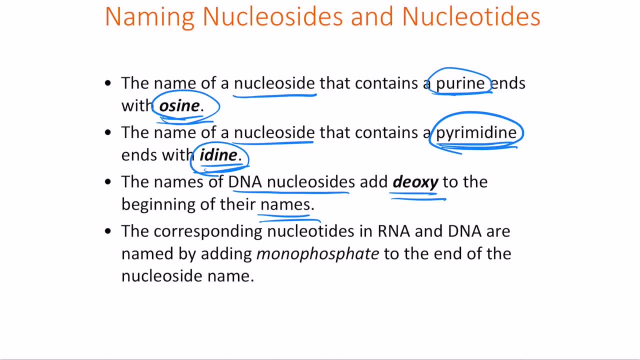 name. If it is not deoxy, we generally write it as generally a general structure. So the addition only comes in when it is a nucleoside of a DNA. Now the corresponding nucleotides in RNA and DNA are generally named by adding a. 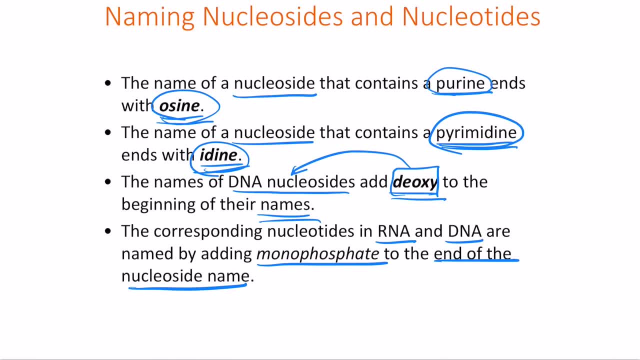 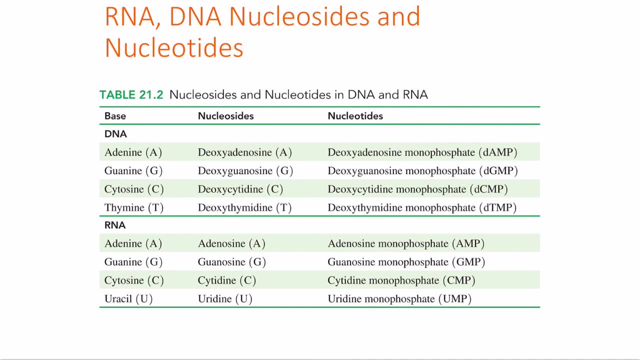 monophosphate to the end of the nucleoside name. So the monophosphate here is the one that ends up creating the final name for the nucleotide. So if the base is adenine, the nucleoside is deoxyadenosine for DNA and the 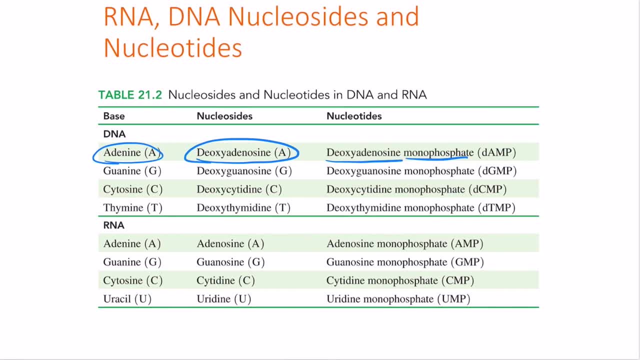 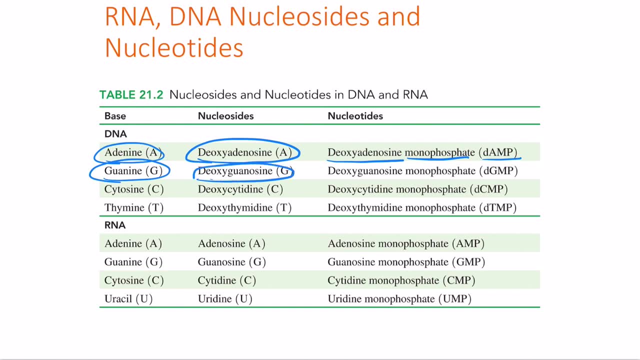 nucleotide is deoxyadenosine monophosphate, So we write it as D-AMP. so the D here represents that it is for the DNA. If it is guanine, you get deoxy guanosine. The nucleotide is deoxy guanosine monophosphate. So this way you also get the 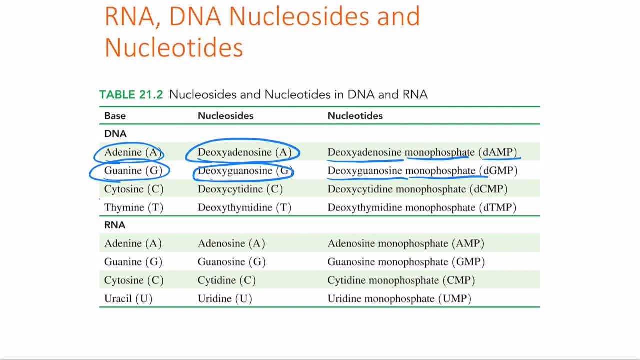 same for C and T In RNA. the only difference is that there is no D. Everything else is the same, but we do not have thymine. but in place of thymine we have uracil. Uracil becomes uridine and uridine monophosphate. 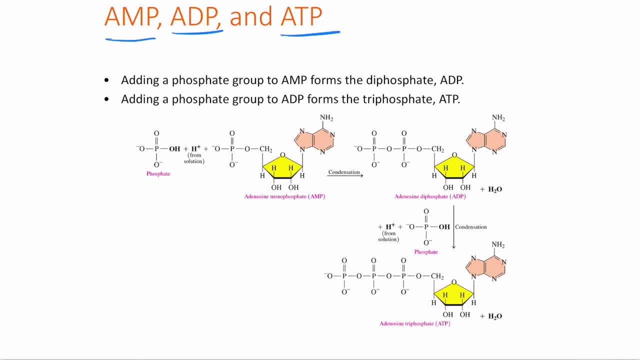 Now let's discuss AMP, ADP and ATP. AMP is adenosine monophosphate, ADP is adenosine diphosphate. ATP is adenosine triphosphate. Now, under condensation processes, the adenosine monophosphate can add itself to. 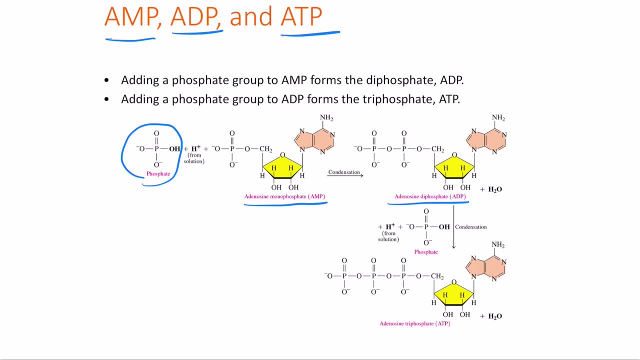 a phosphate, resulting in the formation of an adenosine diphosphate, and further condensation results in the formation of a more powerful and more energetic adenosine triphosphate. So this is the main molecule that is involved in the formation of many of the structures or many of the molecules in your own body. 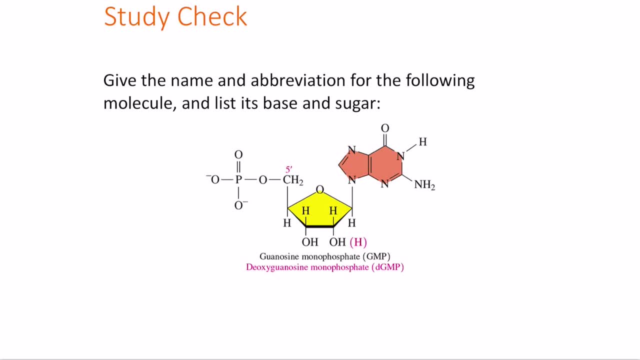 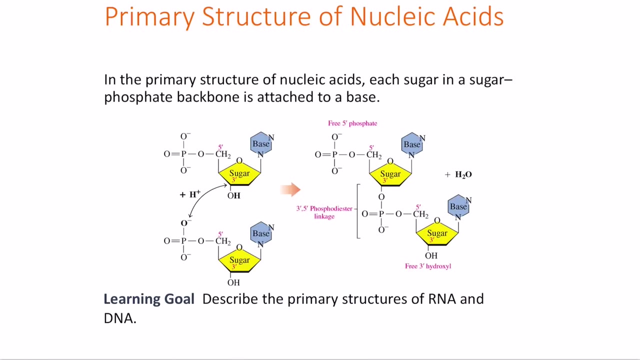 So they are asking you to here. so start to pause the video here and try to solve this problem. So give the name and abbreviation for the following molecule, and it states base and sugar. Now let us talk about the primary structure of nucleic acid. So the primary structure involves: 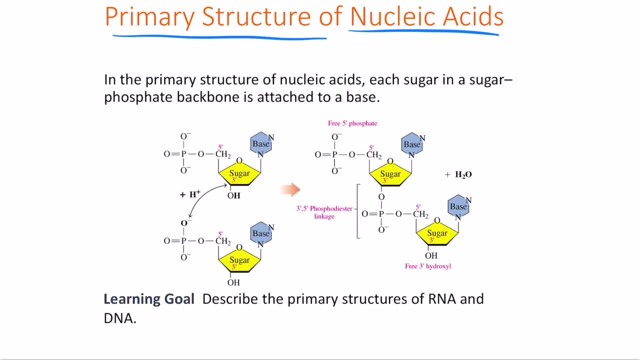 the formation of a phosphodiester bond. So the phosphodiester bond forms between the third carbon, the oxygen connected to the third carbon, and the phosphate group attached to the fifth carbon of the next sugar. So this 3, 5 phosphodiester linkage is the main reason why DNA in itself. 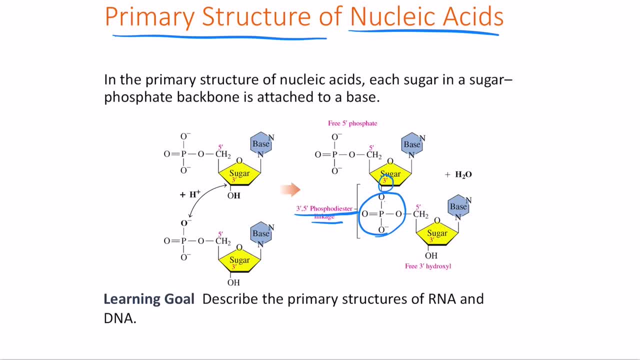 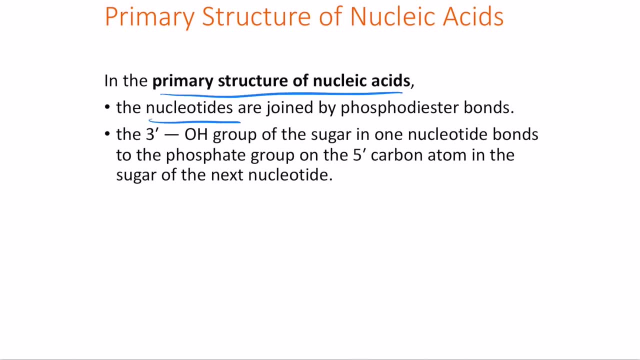 nucleic acids in themselves actually can create a linear polymeristic chain. So the primary structure of nucleic acids involves: the nucleotides are joined by the phosphodiester bonds, So the 3 prime of OH, of the sugar, And one in one nucleotide bonds to the phosphate group of the fifth carbon in. 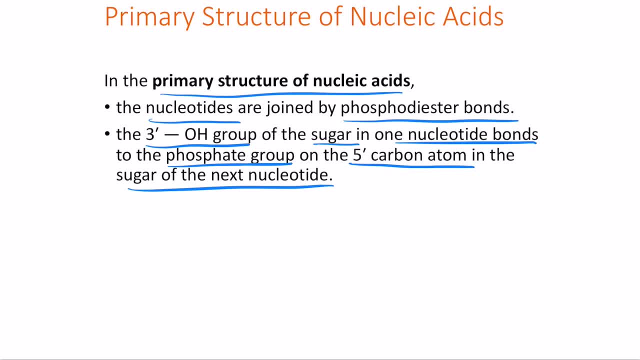 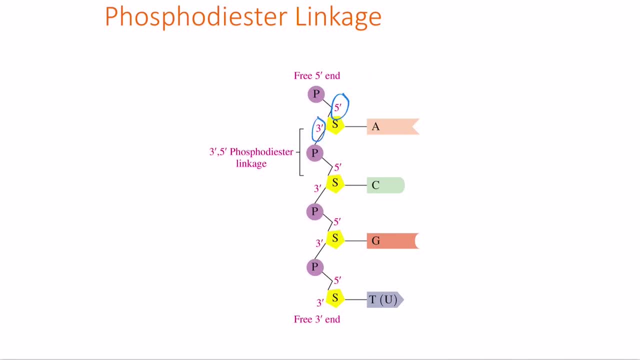 the sugar molecule. Remember that here it is the third 3 prime OH group to the phosphate group of the fifth prime carbon. Now this 3 prime 5 prime bonding is what results in the formation of this phosphodiester linkage. So this is: 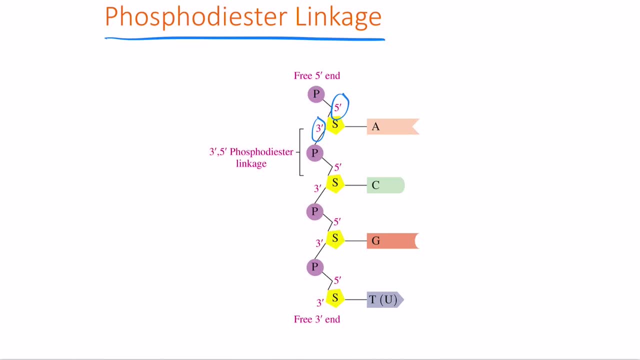 the. this is one of the main important bonds that results in the creation of the DNA. So it's always remember that one end you have a free 5 prime end and on the other end you have a free 3 prime end. So whenever we write DNA structures, 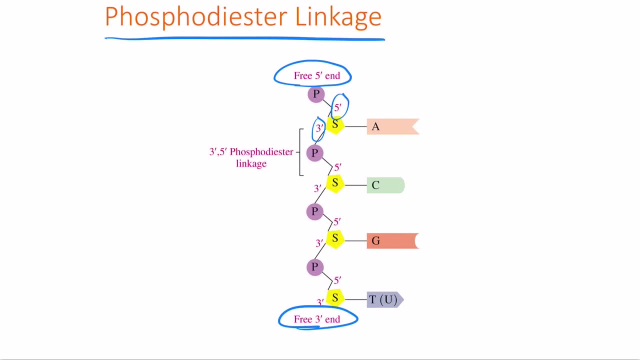 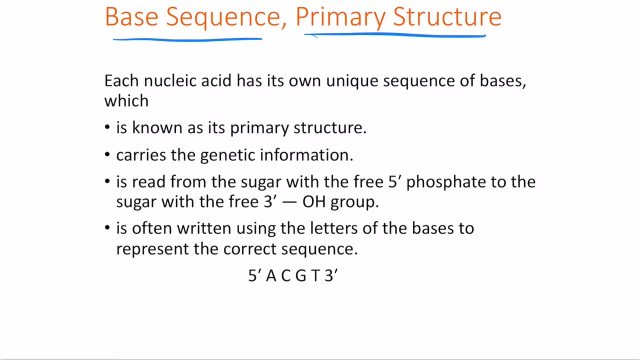 we always write from 5 prime to 3 prime and in reverse we write 5 prime to 3 prime as well. So the base sequence here is the primary structure. So each nucleic acid will have its own unique sequence of bases, which is known as its primary structure. And this is the primary structure. 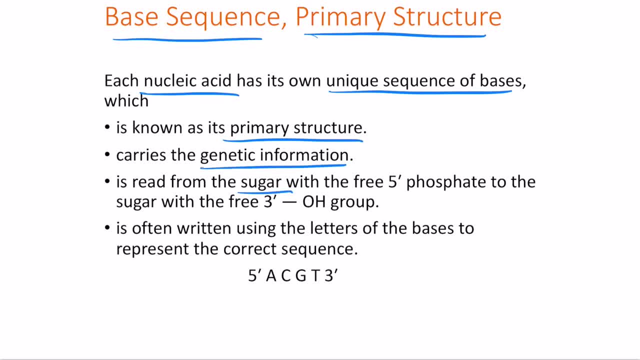 that carries the genetic information. Now it's generally read: from the sugar with the free 5 prime phosphate to the sugar with the free 3 prime phosphate. So it's often written using the using the letters to the bases that represent the sequence. For example, we write 5 prime, ACGT, 3 prime. So we write always from 5 prime to 3. 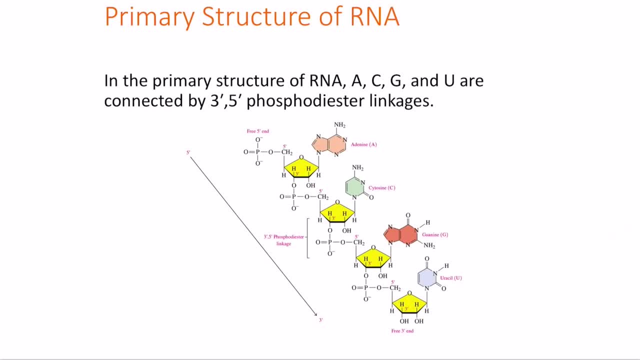 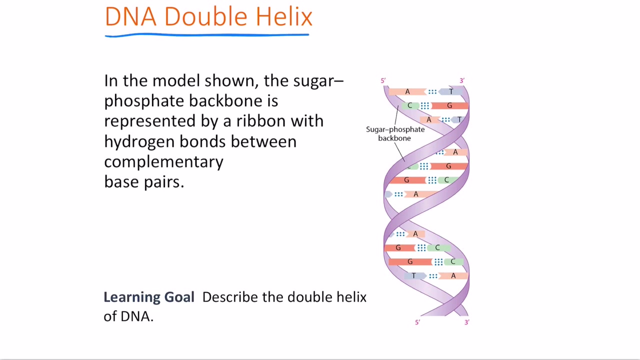 prime whenever we write the primary structure of a genetic sequence. So pause the video right here and try to determine well, what is the from 5 prime to 3 prime. what is the structure here? and try to write it this way. Next is the DNA double helix. So the DNA double helix here is involves the formation of a 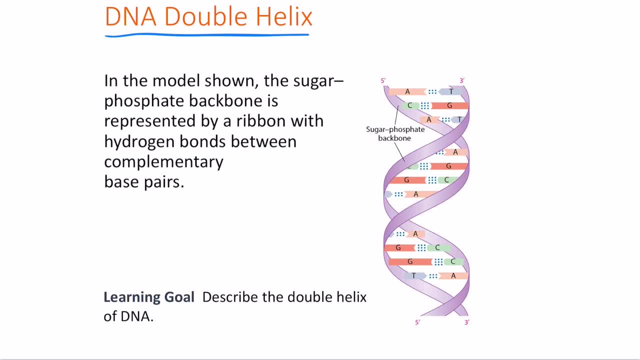 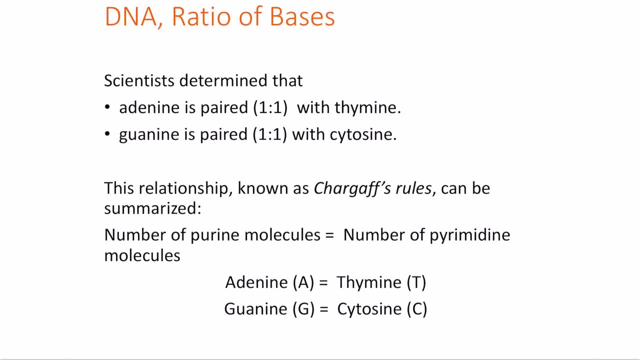 hydrogen bond between the nitrogen bases, between the, between the nitrogen bases that are present on the 1 prime carbon. So what happens here is that it is determined that the adenine is. adenine is generally pairs with thymine in DNA. Guanine also pairs with cytosine in 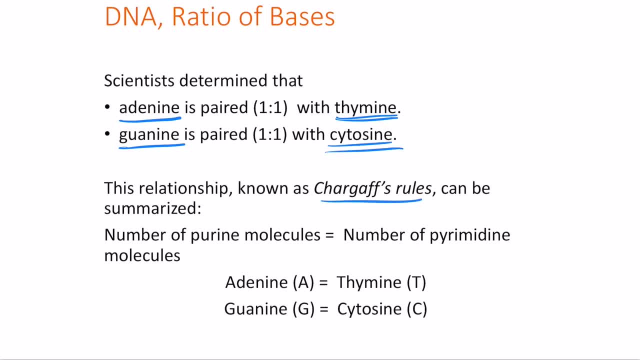 the DNA. So this is generally called the Chargaff rules, which can be summarized as that the number of purine molecules should be equal to the number of pyrimidine molecules. It should always be in a one to one ratio. So here A always pairs with T, G always pairs. 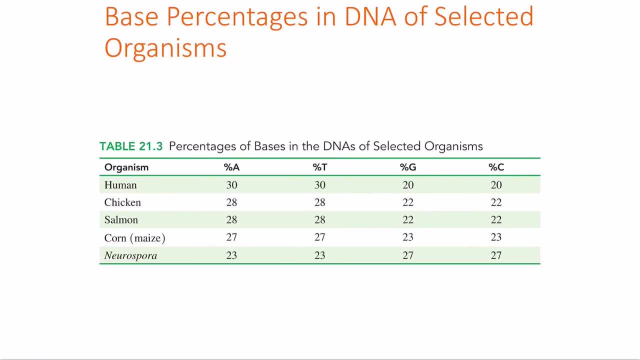 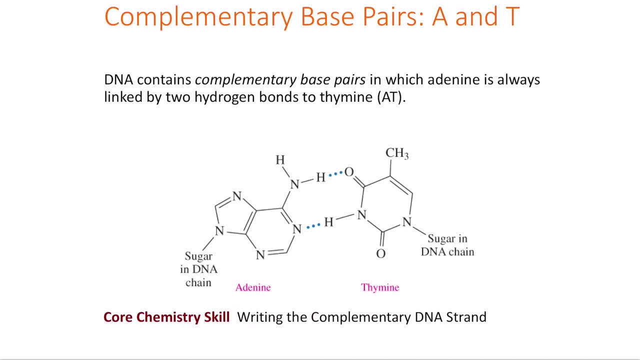 with C. So these are percentage of bases in DNAs of selected organisms. Notice that humans have one of the most highest percentage of bases in DNAs, followed by other organisms. Now the bonding here is a hydrogen bond. This is a hydrogen bond. This is a hydrogen bond. 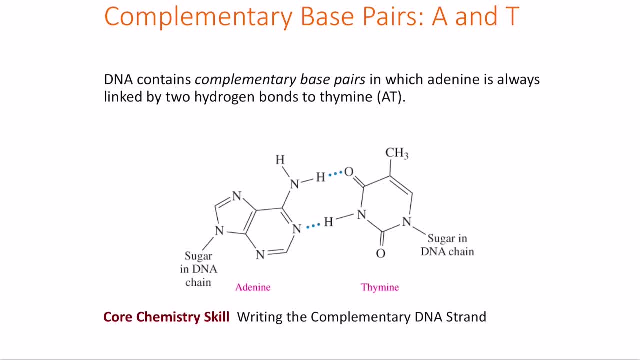 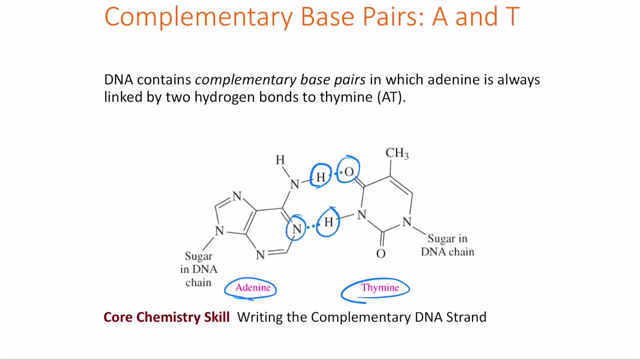 thymine and nitrogen on adenine and hydrogen on thymine. So Ate involves two hydrogen bonds. So Ate formation involves two hydrogen bonds And these are what we call complementary bonds. we call complementary base pairs because they are always going to be bonding with each other. 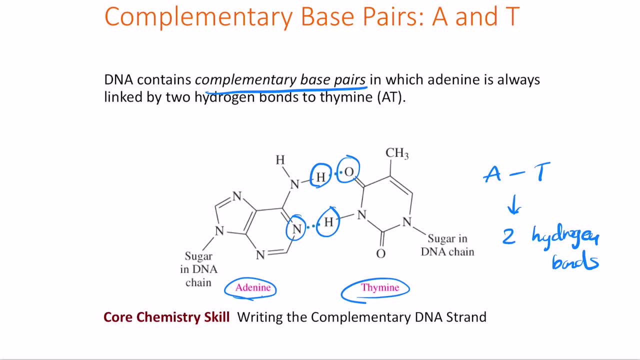 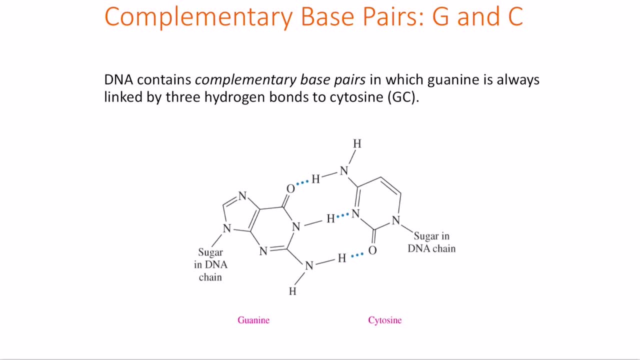 they cannot bond with another structure. for example, adenine cannot bond with cytosine or adenine cannot bond with guanine. so when you take guanine and cytosine, guanine and cytosine, these are also complementary base pairs. so here it involves three hydrogen bonds. so gc involves 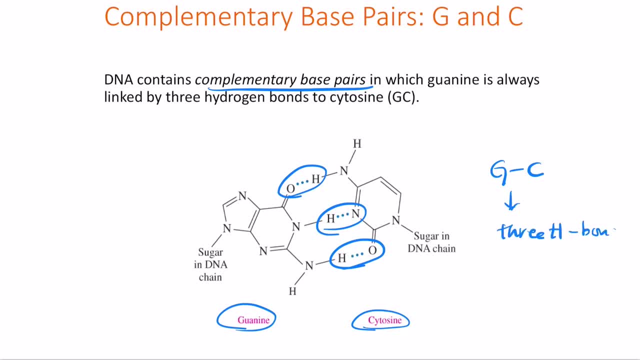 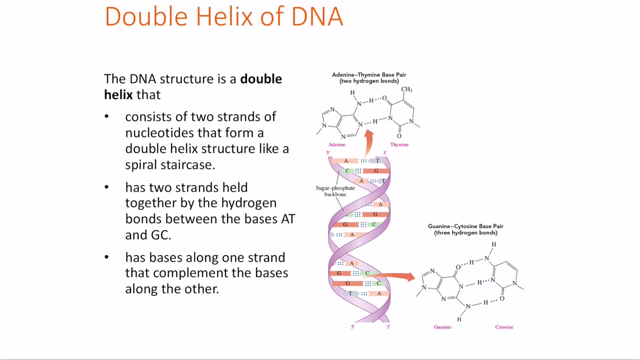 three hydrogen bonds. so gc involves formation of three different hydrogen bonds. so the double helix of dna is created by first the primary structure, where we get five prime to three prime on one of these, one of these helices, one of the structures, and five prime to three prime. 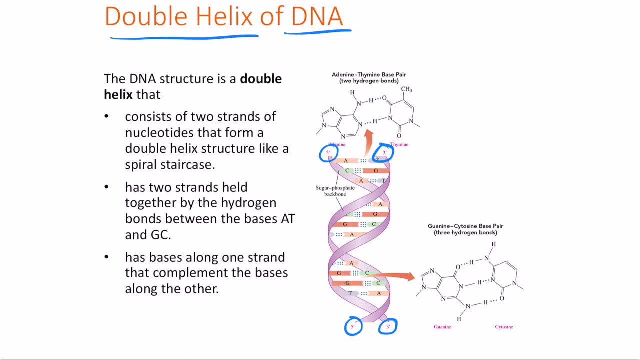 is the primary structure, three prime on the reverse, on the other side. so one complements the other and the complementing dna helix structure is formed because of the hydrogen bonds that form between the structures here, and these hydrogen bonds are the ones that result in the formation of a double helix structure. 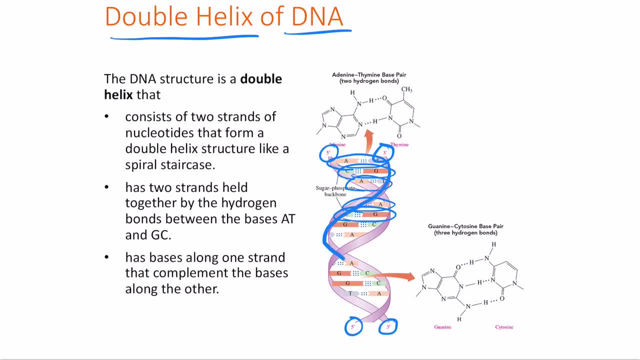 so you have: on outside you have the sugar phosphate bonding and on the inside you have the hydrogen bonding between the nitrogen bases. so the dna here enters into a double helix structure. so it contains two strands of nucleotides that are forming a double helix structure like a spiral staircase. so it generally has two strands held. 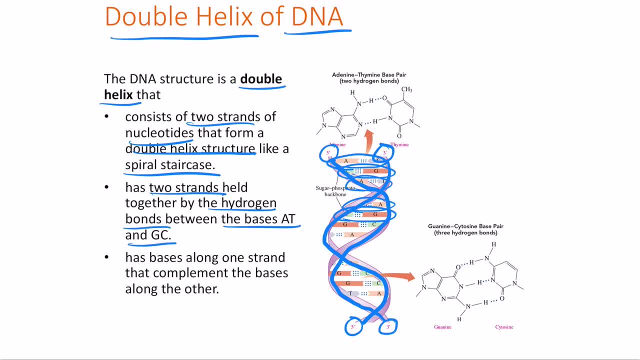 together by hydrogen bonds between the at, between the bases at and gc, and it also has bases along one strand that complement the basis on the other. so remember that a always bonds with t and g always bonds with c. for example, if you have five prime: a, c, g. 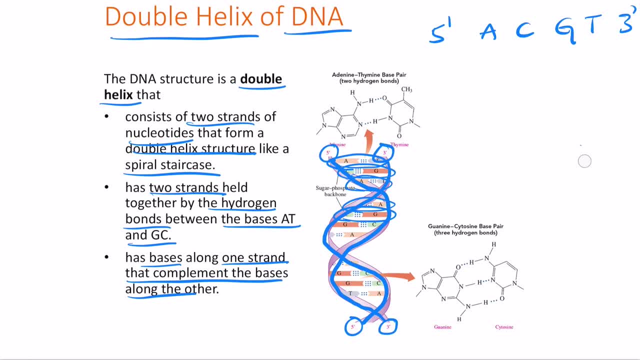 d, t, three prime on reverse side. always it has to come from the complementary side, so it will become phi prime t bonds with a, g bonds with c, c bonds with g, a bonds with t and three prime. so remember that this bonding should always be with a complementary pair, so one. 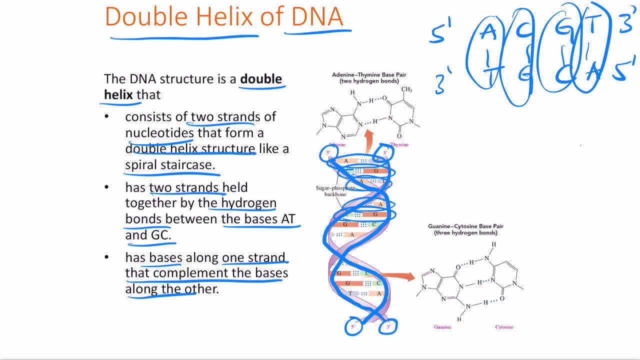 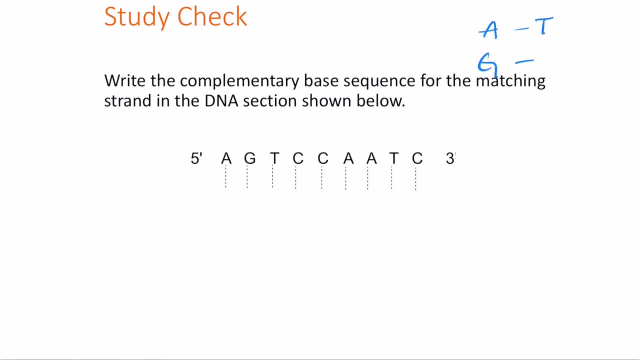 one strand complements the other strand. so this is the idea behind the structure here. so try this one. pause the video right here. remember that a should bond with t and d, G should bond with C. So pause the video here and try to determine the complementary chain. 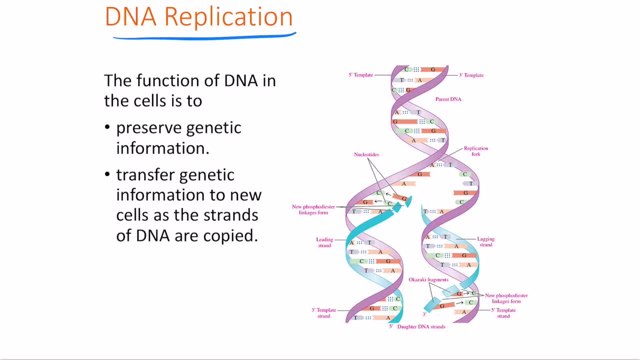 Next let's talk about DNA replication. So the function of the DNA is to, in the cells, is to preserve the genetic information. So the way it can preserve it is to transfer the genetic information to new cells, as the strands of DNA are copied, So it basically copies the DNA. so 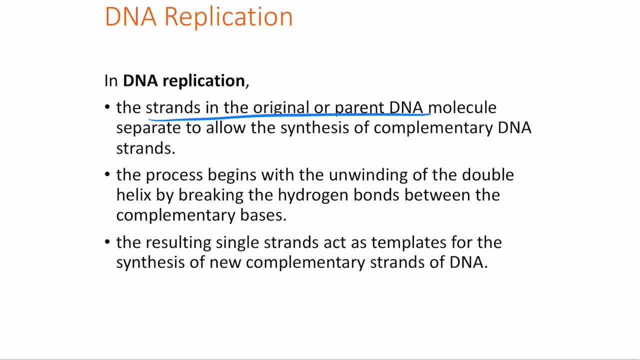 the strands in the original DNA or the parent DNA separate to allow the synthesis of a complementary DNA strand. So this process first begins with unwinding of the double helix structure by breaking down the hydrogen bonds between the complementary bases, and then the resulting single strands act as templates for the synthesis of new complementary strands of DNA. So this here: 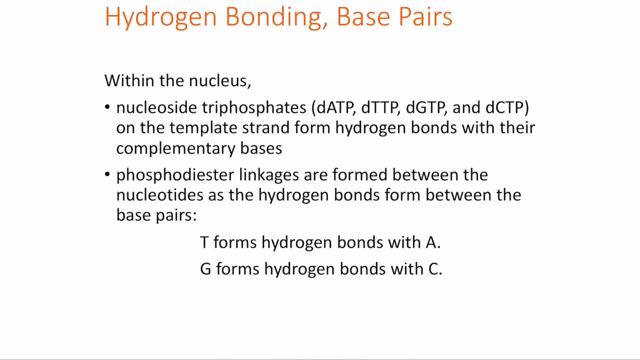 is the process of DNA replication, where it replicates itself to create copies of itself, So within the new nucleus. so you have nucleotide triphosphates on the template strand from hydrogen bonds with their complementary bases and the phosphodiester linkages are formed between the nucleotides as 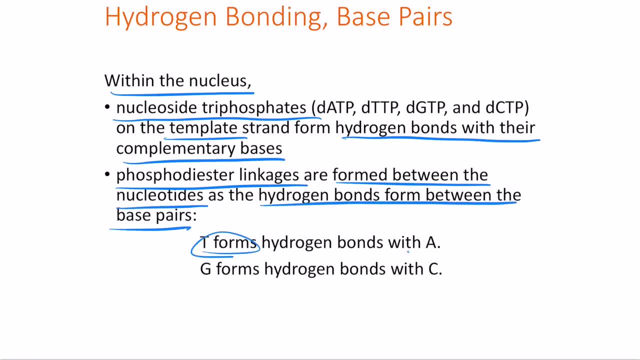 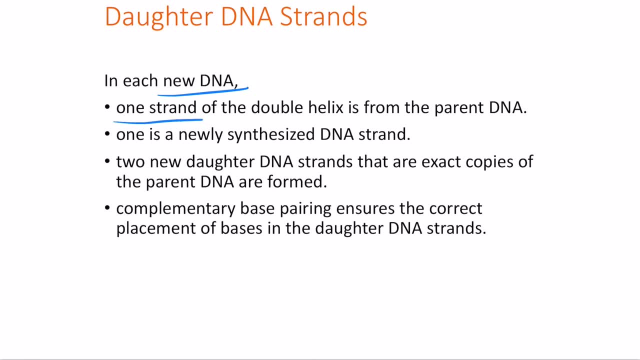 the hydrogen bonds form between the bases. Always remember: the T forms hydrogen bonds with A and G forms hydrogen bonds with C. So in each new DNA strand you will have one strand of double helix from the parent DNA and one is the newly synthesized DNA strand And you have two new. 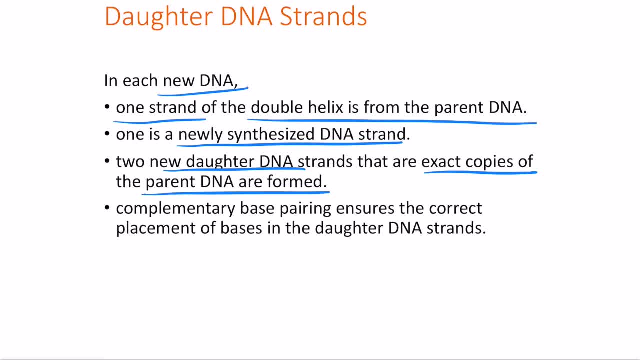 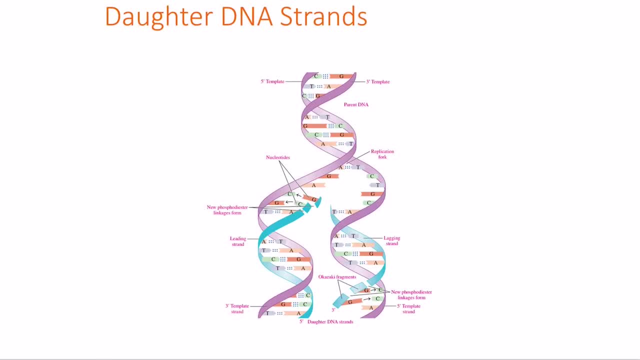 that are exact copies of the parent DNA that are going to end up forming, And a complementary base pairing ensures that the correct placement of the bases in the daughter DNA strand always occurs. So this is the process of DNA replication. Now the direction of replication involves 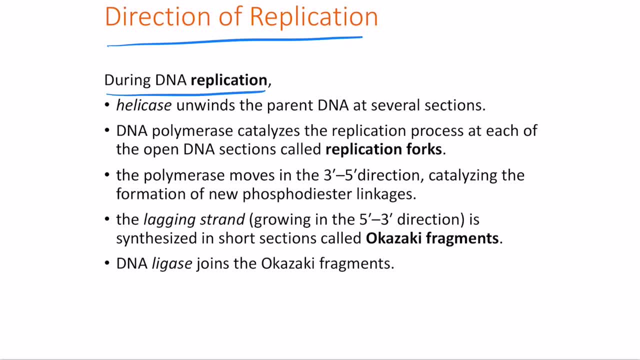 so, during the DNA replication, you have an enzyme that creates this replica or replicas. we call it helicase, so he will. it is the enzyme that unwinds the parent DNA at several sections. So this is that, you see. So this is the enzyme that creates the replica, replicas. we call it helicase, so helicases the enzyme that unwinds the parent DNA at several sections. So this is. The second is theELIOnis ie trans hocesituomепiol lieberen. requirements are different if you are going to make a combination of DNA and t hearlikase or responsible to 993c肌酸ar weeks today. if you cared not to. 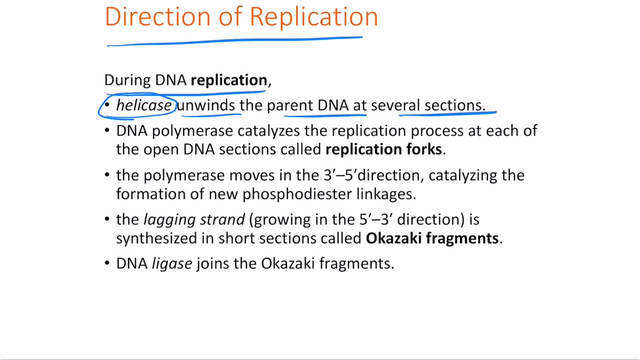 sections. so this is the one that envines the parent dna and the dna polymerizes the enzyme that catalyzes the replication process. so think of it like a replication forks: it starts cutting them up and attaching them to new strand. now the polymerase here moves in three to five direction. 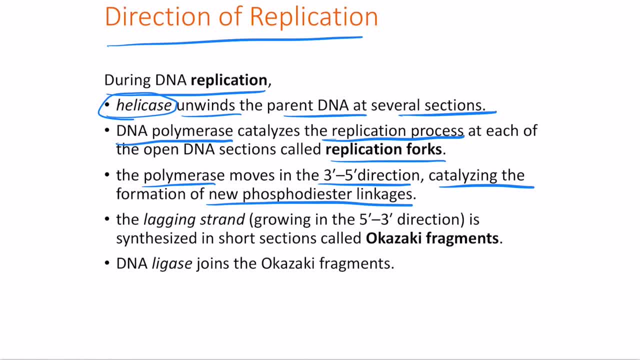 three prime to five prime direction, catalyzing the formation of new phosphoester bonds. you will get two types of two strands. one is the leading strand, the other is the lagging strand. leading strand is a direct process where it attaches itself but one ends up becoming a lagging. 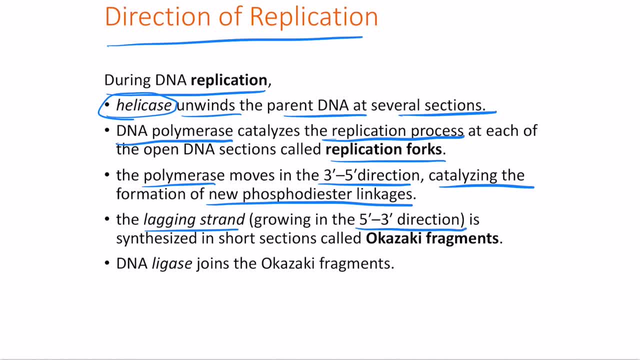 strand because it grows in the reverse direction. these types of sections are generally synthesized in short sections. we call them okazaki fragments. so for that okazaki fragments, we use another enzyme called dna ligase to join the okazaki fragments to create the final structure of the dna. 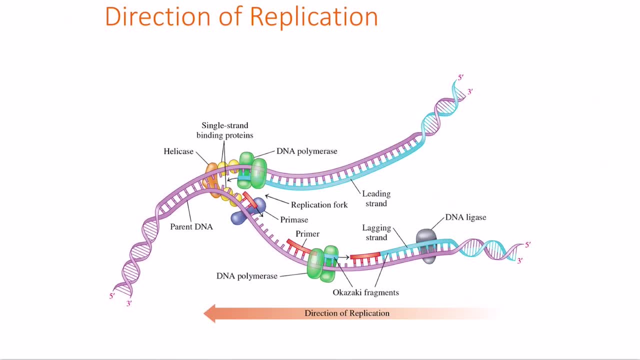 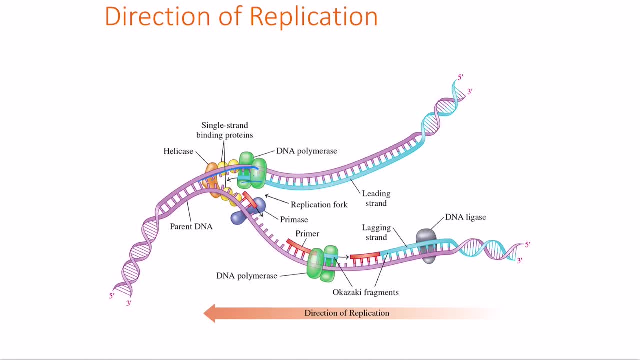 complementing the base plate to create the dna. but you have one side it could. it is basically taking from five prime end to three prime end. but here it is. it's taking it from three, five prime to three prime, so it's in the reverse direction. so what we'll have to do is that it will create a 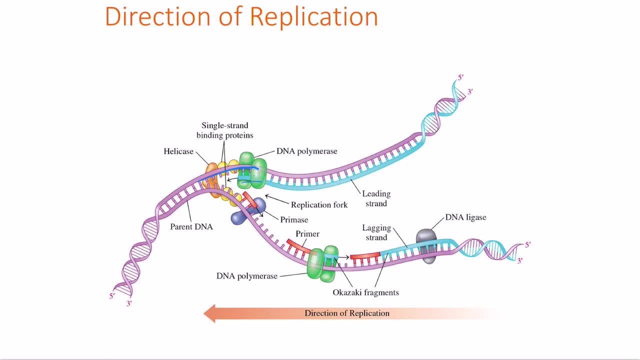 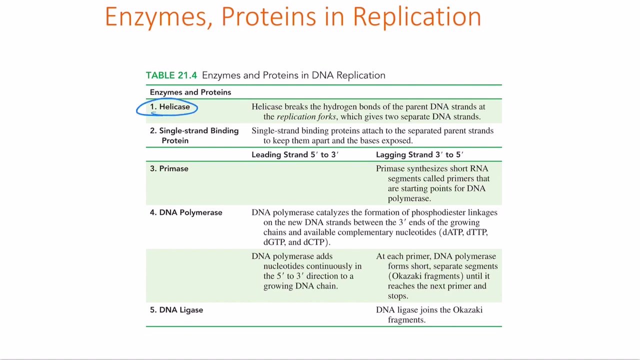 lagging strand. so the lagging strand basically attaches up, attaches parts of it. so the dna ligase fills up the gaps that the dna polymerase cannot fill up during the process. so what are the enzymes involved? first is the helicase enzyme. it involves the breaking of the 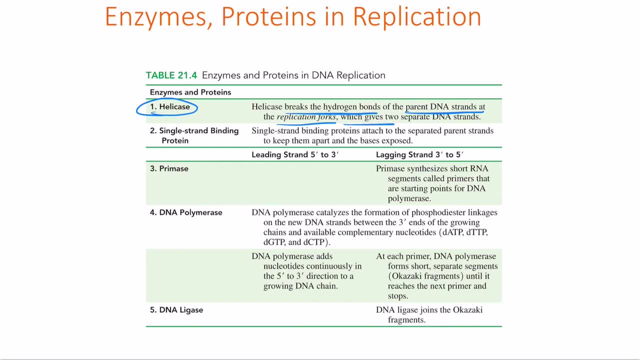 hydrogen bonds of the two parent dna strands at the replication. fourth, which gives two dna, two separate dna strands. second is the single strand binding protein, which is the one that attaches to the separate parent strands to keep them apart, and the base is exposed. so next you have primase. 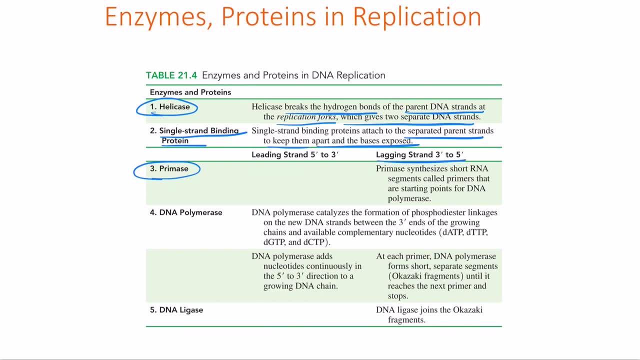 primase is involved in the lagging strand. it is basically a single strand binding protein synthesizing short dna rna segments, called primers. they become the starting midpoints for the dna polymerase. so the dna polymerase involves the catalysis of the formation of the phosphodiester. 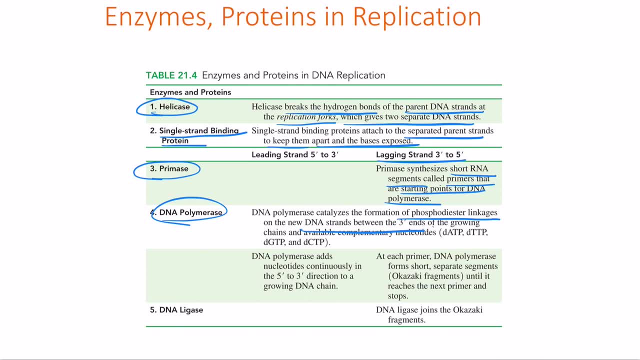 bonds between the new dna strands of the three prime to the other complementary nucleotides. now dna polymerase adds nucleotides continuously to five to five prime to three prime. but at each primer on the lagging strand dna polymerase will form short, separate segments. reaches the 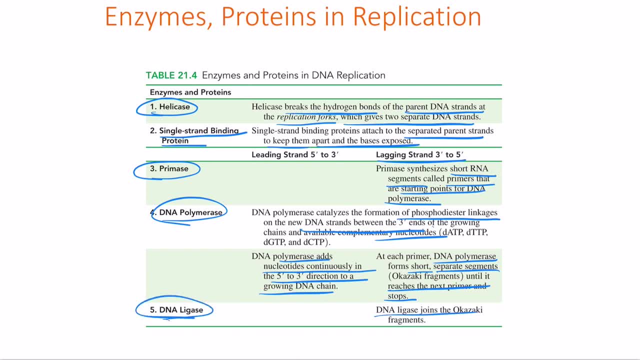 next primer at the stop. so dna ligase is a single strand binding protein, which is a single strand binding protein, which is the one that basically create, basically checks the for a lagging strand and make sure that it bonds the lagging strand to to not it be separate. so pause the video, right. 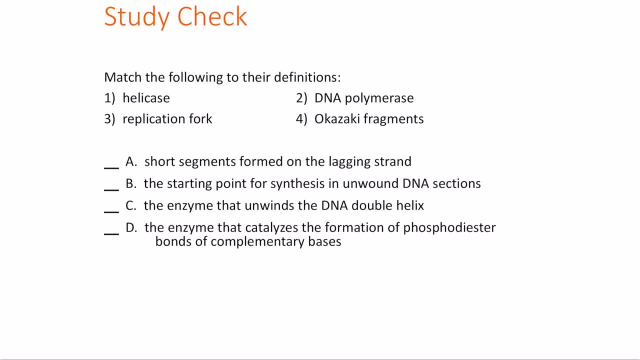 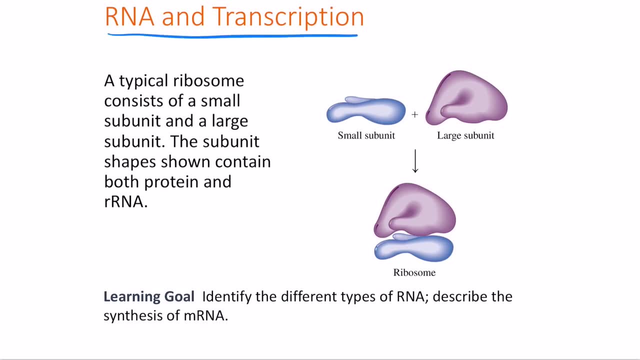 here and try to answer these questions. next let's talk about the next process, which is transcription. so a typical ribosome in general contains a small subunit and a large subunit of ribosomes. so the subunits generally are the ones that create the final protein. so let's start with rna and dna. 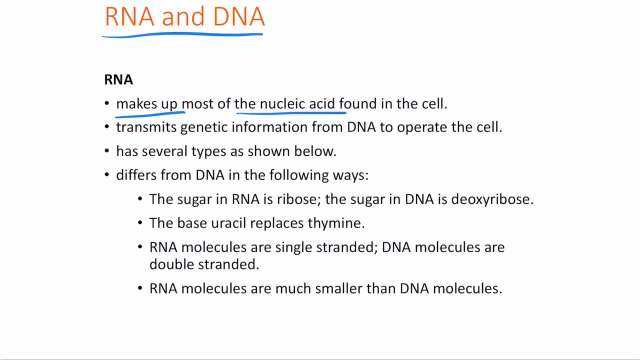 so rna here is generally the one that makes up most of the nucleic acid that is found in the cell. so rna here transmit the genetic information from the dna to operate the cell. so think of rna as specific set of instructions that are taken from the dna to create entities in the cell. 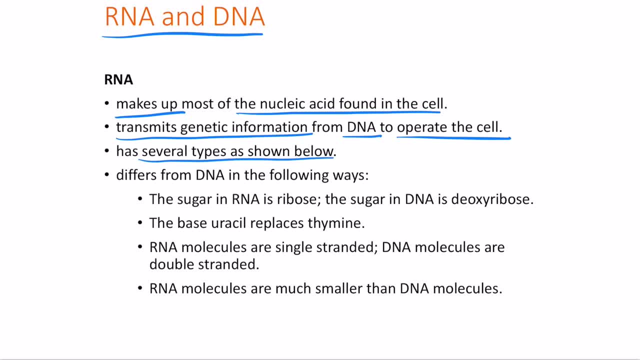 so there are several types. so they also differ from dna in the following ways. first, the sugar is a ribose and the sugar in dna is a deoxyribose, so the base uracil replaces thymine and the rna molecules are single standard and dna molecules. 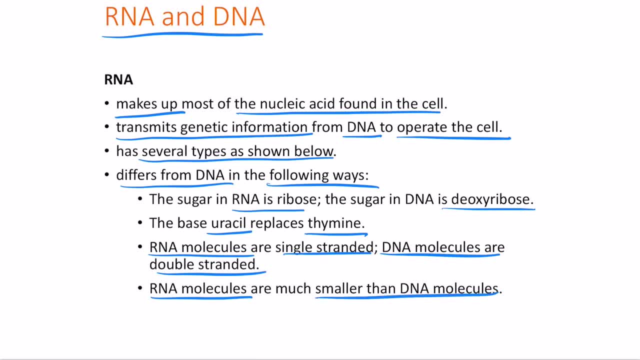 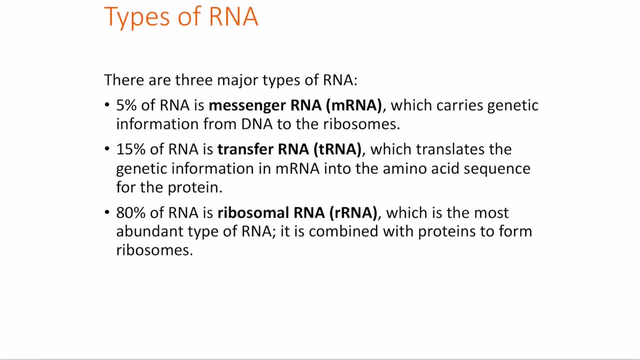 are double standard and rna molecules are generally much smaller than dna molecules. remember the first thing, that it's a single standard one, which means that it is really small as well, as these are not that that large in comparison to dna's. now there are three type. 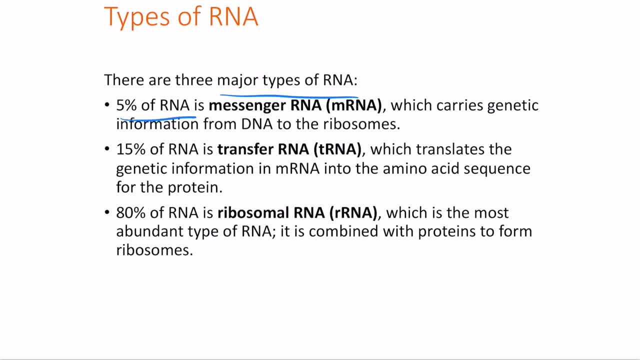 three major types of dna. five percent of the dna molecules are single standard and the other three are the same type of dna, which is the one that is used to carry genetic information from dna to the ribosomes. 15 percent of the rna is transfer rna, which is trna, which translates the genetic 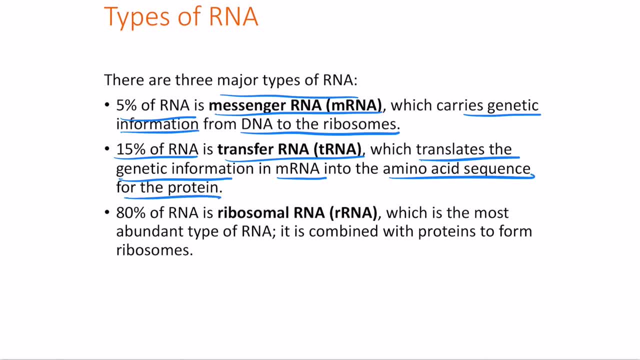 information in the mrna into an amino acid sequence for the protein. 80 percent of the rna is ribosomal rna or rrna, which is most of the abundant type of rna. it is the one that combines with proteins to form ribosomes. let's start with trna, so trna can be. 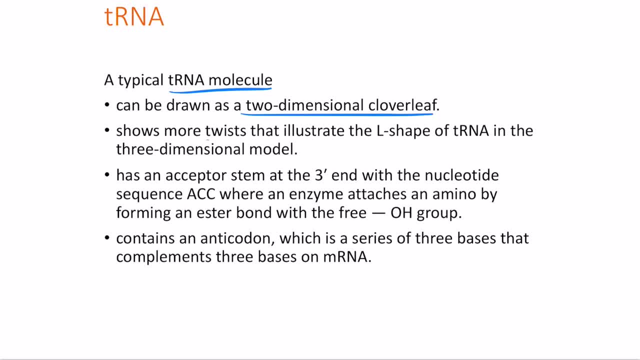 drawn as a two-dimensional clover leaf so it shows more twists than illustrated. the l shape of the trna is in the three-dimensional model, so trna has an acceptor stem at the three prime end with the nucleotide sequence acc, where an enzyme attaches by the amino acid forming the ester. 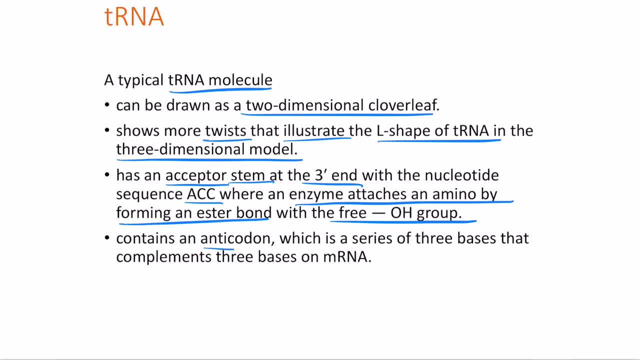 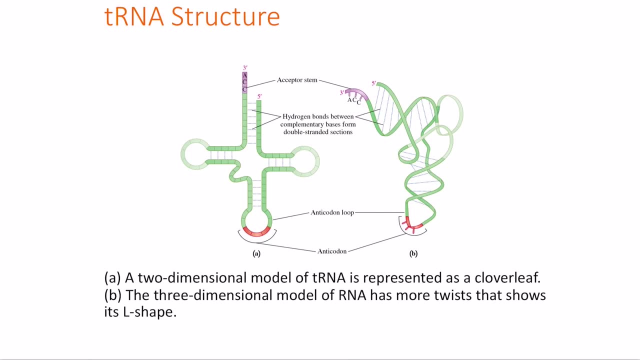 bond to free the oh group. so it generally contains what we call an anticodon, which is a series of three bases that complements the three bases of the mrna. remember that the transcription process always starts at a. so this is the structure of a trna in general and it has much more twist than it is shown. 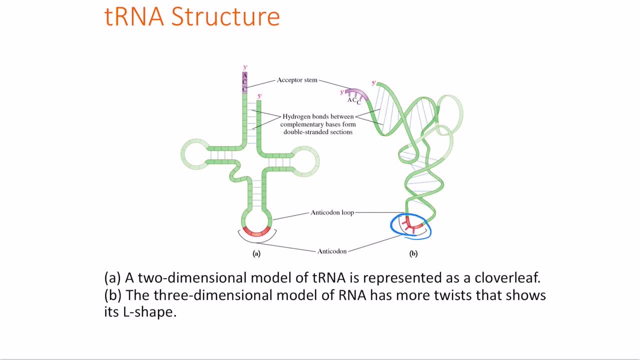 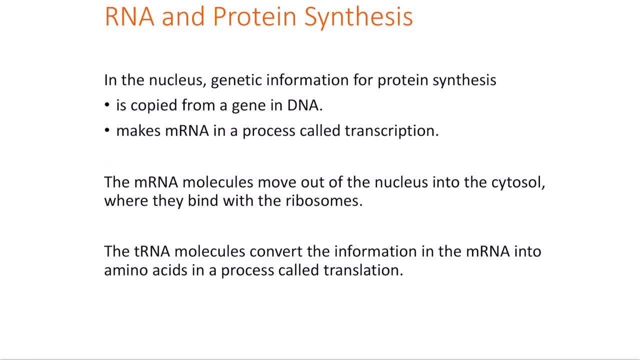 here, and on one end you have the anticodon loop and on the other end you have the acceptor stem. acceptor stem is the point where the transcription starts. so what is the process of transcription here? so in the nucleus we are basically what we are doing in the transcription. 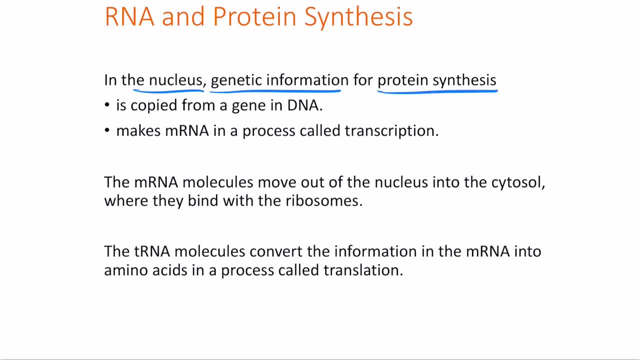 is, we are converting the genetic information in the dna protein. so what is going to first happen is that first the data, that the genetic information needed from the gene, is copied from the DNA and in the process we make mRNA. this process of converting DNA into mRNA is called transcription. 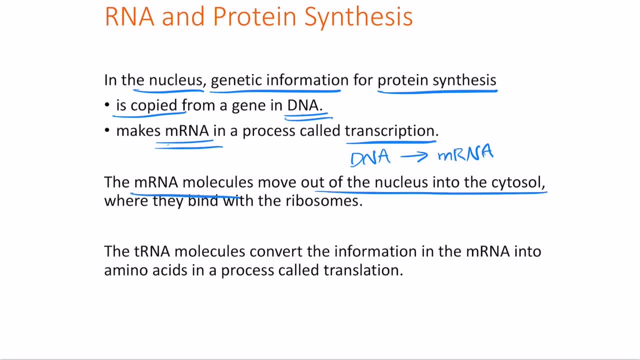 So here the mRNA molecules move out of the nucleus into the cytosol where they bind with ribosomes, and ribosomes are the materials that convert the mRNA into proteins. So this process of converting mRNA into proteins is called translation. So remember that we discussed in total three processes: replication, where DNA copies itself. 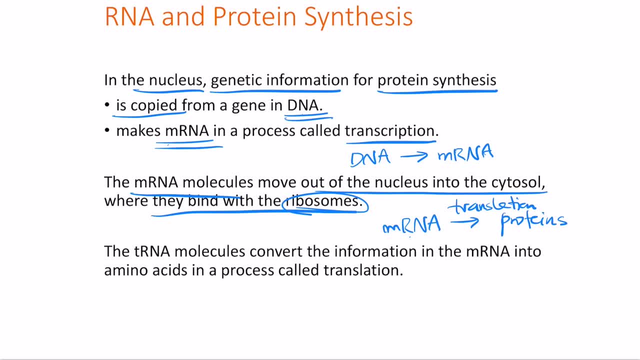 and creates two parent, two daughter chains, two daughter structures: transcription, which is the conversion of DNA into mRNA, And translation, which is the conversion of mRNA into proteins. So the mRNA here is the process. the transcription, the process of replication occurs inside the 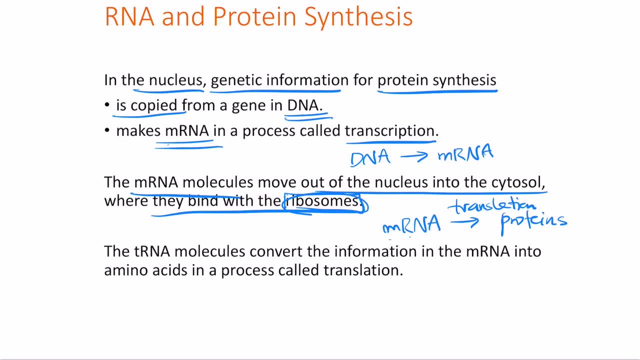 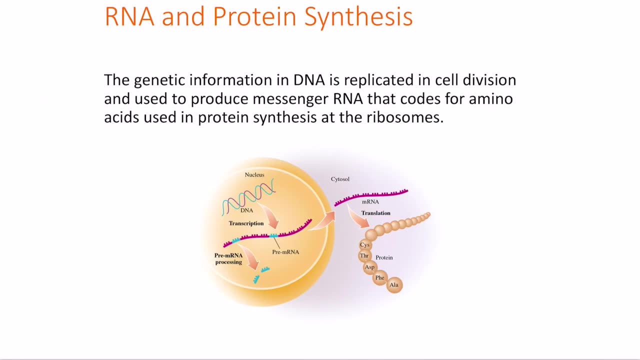 nucleus. transcription also occurs inside the nucleus, but translation occurs in the cytosol outside the nucleolus, Now the tRNA. here molecules convert the information in the mRNA into amino acids in the process called translation. So what will happen first? First the nucleus either replicates itself, and the second process that it can do is transcribe. 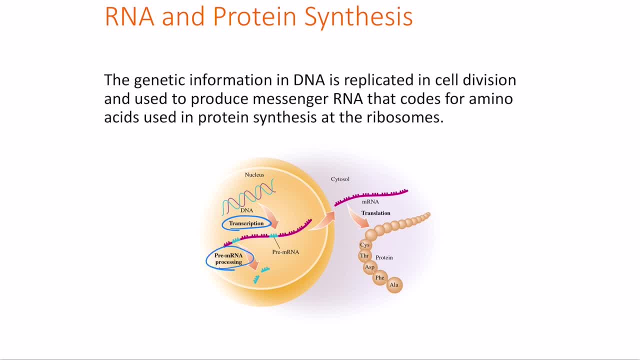 So the transcription process involves the creation of a pre-mRNA processing unit, so where it creates a mRNA, The mRNA then comes out of the nucleus into the cytosol, where the mRNA bonds with the ribosome and the ribosome converts the sequence of mRNA into amino acid sequence and the amino 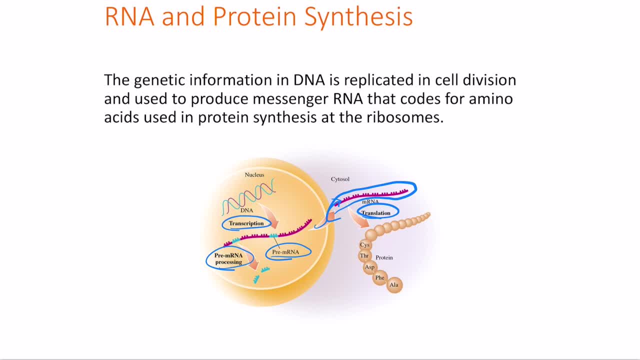 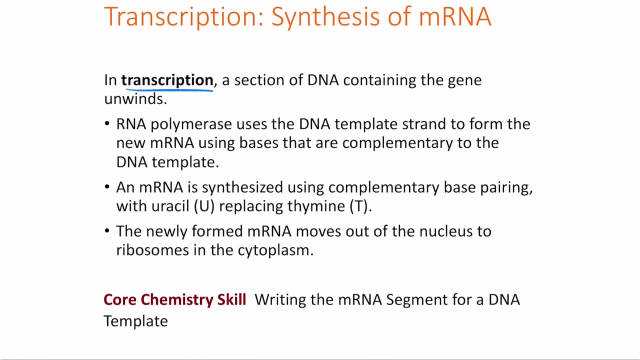 acid sequence creating the process of primary structure of the protein. So remember that translation involves the conversion into primary structure and the structure then evolves to create more complex structures. So in transcription here you are basically taking a section of the DNA containing the gene and we are unwinding it, and the enzyme, RNA polymerase, uses the DNA template strand. 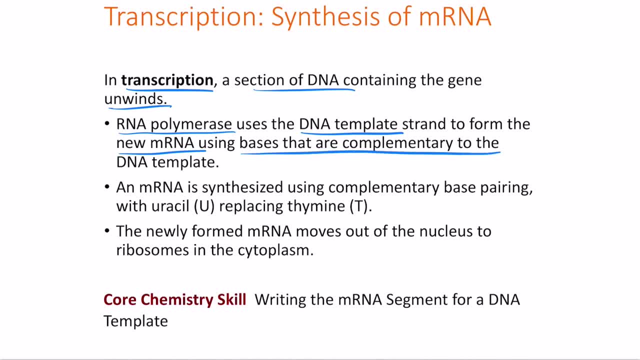 to form a new mRNA using the bases that are complementary to the DNA template. So the mRNA here is synthesized using the complementary base pairing, where we basically use U instead of uracil, instead of thymine. So the newly formed mRNA here first then moves out of the nucleus to the ribosomes in the 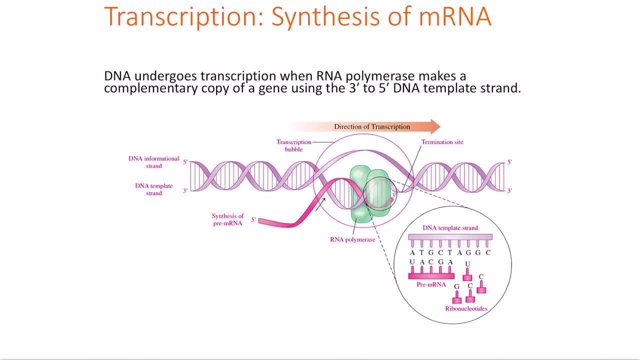 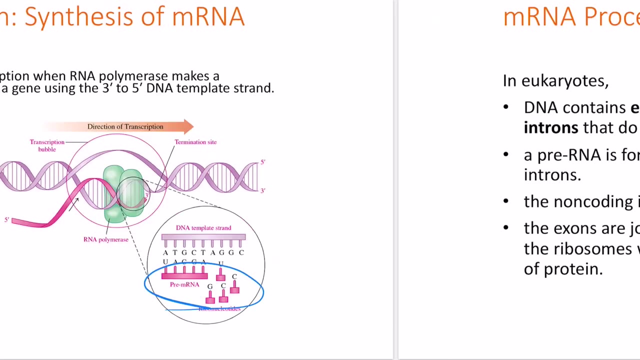 cytoplasm. So basically it cuts a part of the DNA at a part of the strand and then synthesizes the mRNA and then moves out, and then the mRNA then creates the pre-mRNA that goes outside the nucleus, Finally creating the new process for translation. 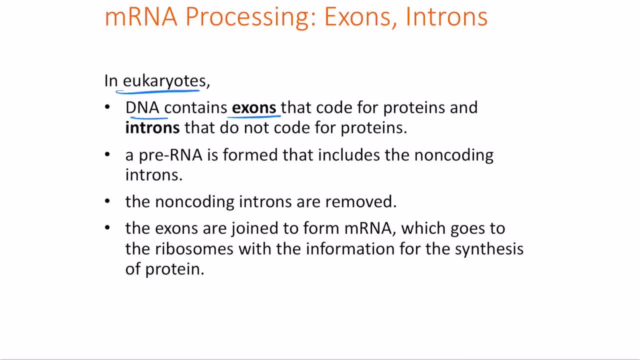 So in eukaryotes the DNA contains exons that codes for proteins and introns that do not code for proteins. So there are two types that are involved. So you have exons and introns. A pre-RNA is formed that includes non-coding introns. 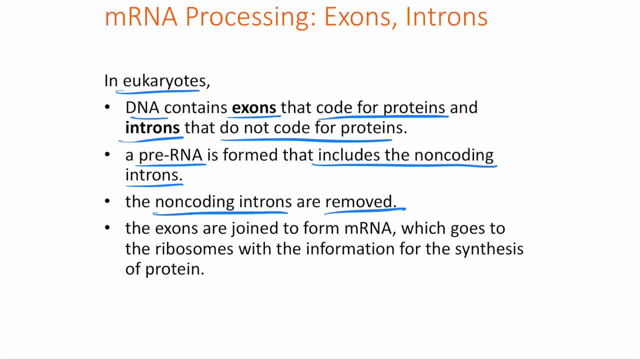 The non-coding introns are generally the ones that are removed. So the exons are joined to form mRNA, which goes to the ribosome, The ribosome with the information for synthesis of the protein. Remember that exons are the ones that are going to end up creating the mRNA, not introns. 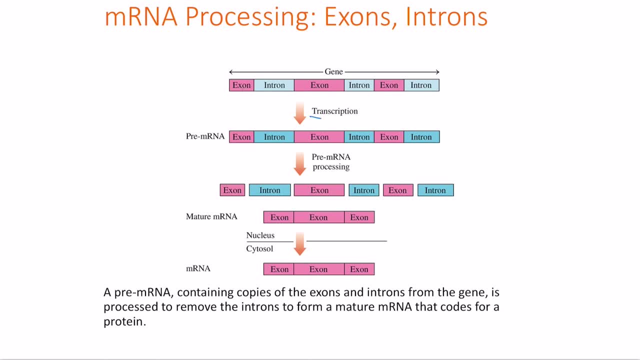 So we basically have exons and introns combined. Finally, during the transcription process, you are basically splitting the structure and finally creating in the pre-mRNA processing place. we remove the introns and finally bond only the exons, finally creating the mRNA strand. So the structure. 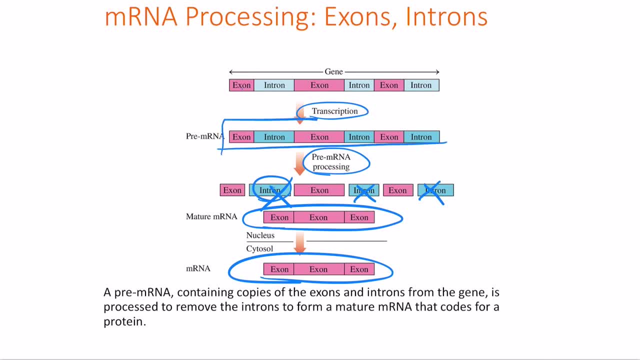 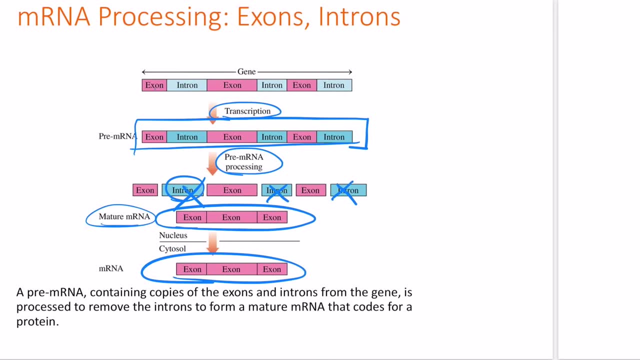 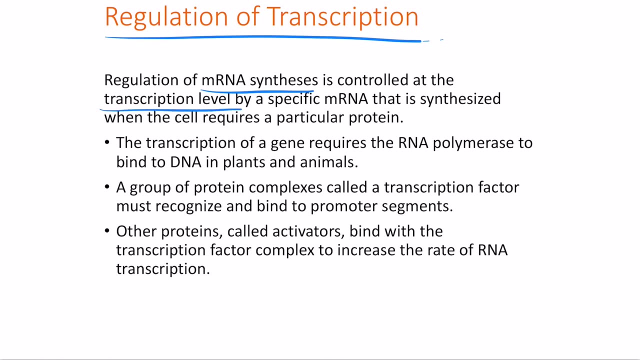 So the structure? So the structure that has exons and introns is called as pre-mature or pre-mRNA, and once the removal of introns happens, we call it the mature mRNA. So how do you regulate the transcription process? The regulation of mRNA synthesis is controlled at the transcription level by a specific mRNA. 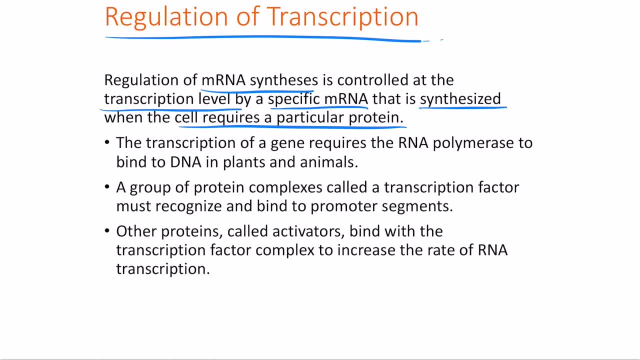 that is synthesized when the cell requires a particular protein. Now the transcription of a gene requires the RNA polymerase to bind to DNA. in plants and animals, A group of protein complexes called as a transcription, As a transcription factor, first recognize and bind to the promoter sequences. 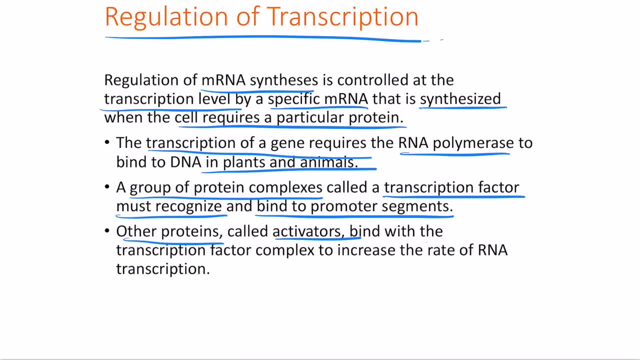 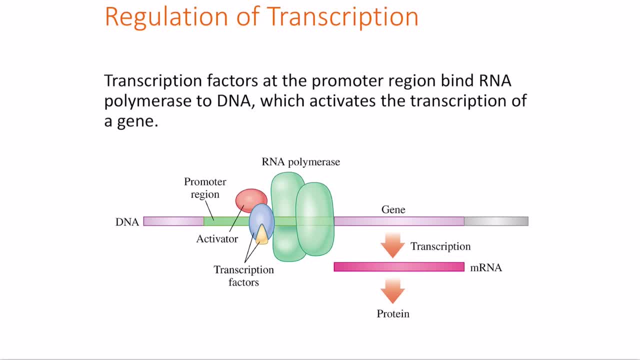 So the other proteins called activators, bind with the transcription factor complex to increase the rate of RNA transcription. So it involves multiple processes. First you have an activator. Activator is the first one that attaches. then you have the transcription factor that attaches. 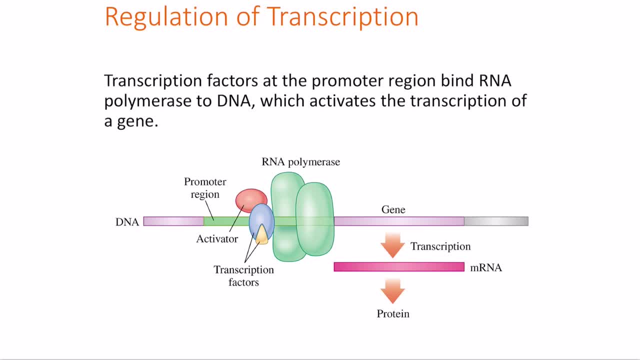 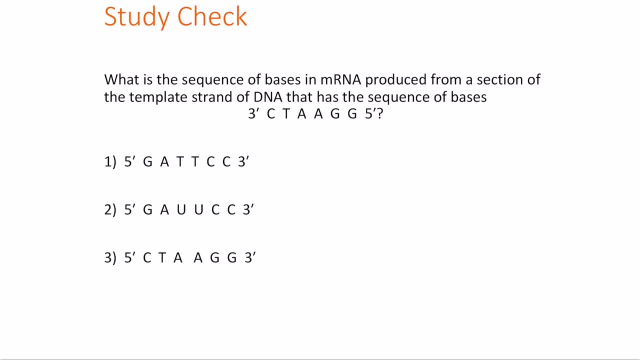 Finally, you have the RNA polymerase that detects the activator and the transcription factor, finally ending up creating the mRNA strand. So that is the process. So that is the process. So that is the process. Now, remember that here also, it involves complementary formation, which means that A here from bonds 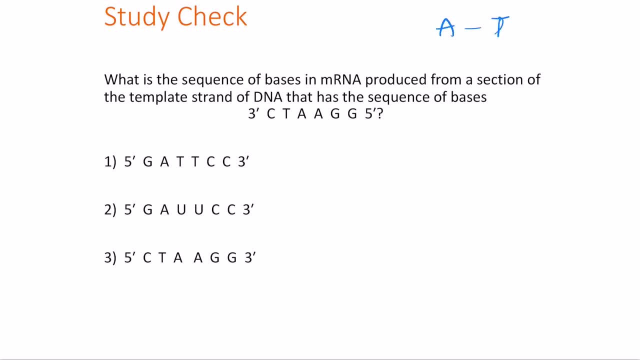 with G. A here bonds with U in terms of the mRNA strand. You have G bonding with C, So use this strand and try to create the template strand of the mRNA. Next, let's talk about the genetic code and protein synthesis. Next, let's talk about the genetic code and protein synthesis. 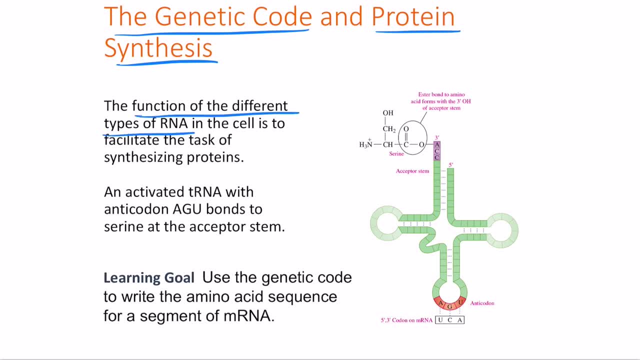 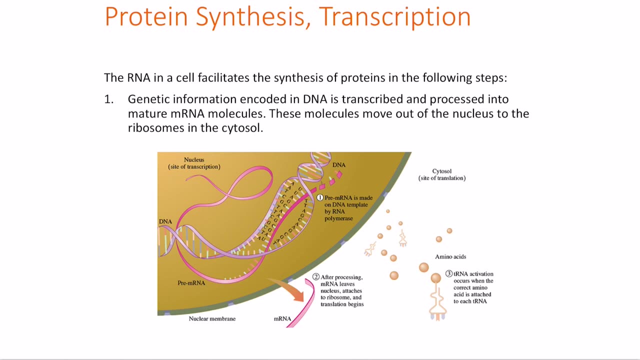 Now, the function of different types of RNA in the cell is to facilitate the task of synthesizing the proteins. An activated tRNA with anti-codon AGU bonds are to serine at the acceptor step. So what is happening here? First, we discuss that there are pre-mRNA and the pre-mRNA splits itself and finally creates. 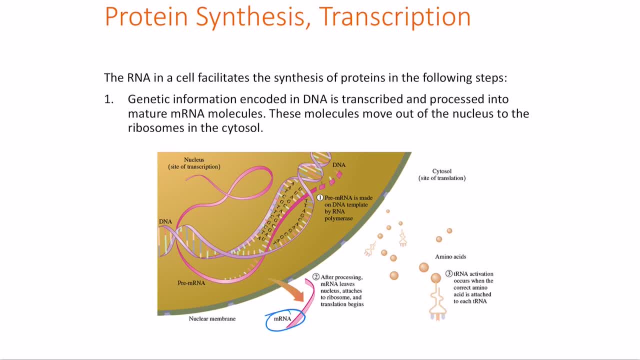 the mature mRNA. So once the mature mRNA comes out of the process here, so the genetic information encoded in the DNA is then transcribed and processed into the DNA. The DNA is then transcribed and processed into mature mRNA molecules and these molecules move out of the nucleus to the ribosomes. 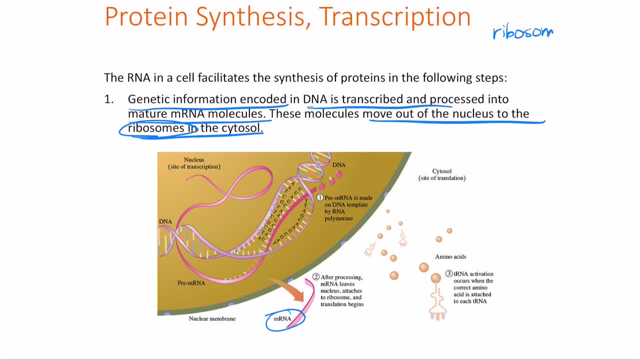 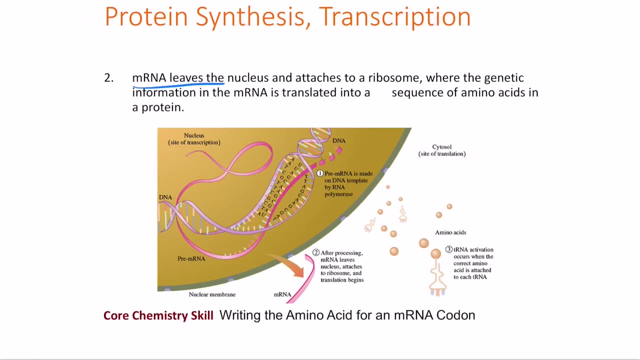 So ribosomes are protein factories, So think of them as protein factories. So these are the structures that these are the proteins that involve the formation of the protein structure itself. So in the second process the mRNA will leave the nucleus. attach us to a ribosome. 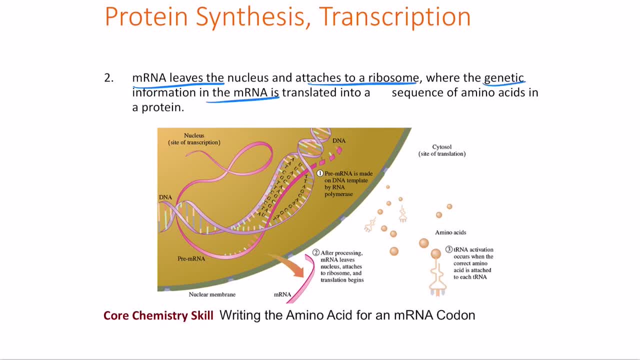 So the ribosome will detect the, will read the genetic information in the mRNA And translate it to create a sequence of amino acids into a protein. So the ribosome here is going to convert the mRNA's message into a sequence of proteins. We call it the primary structure. 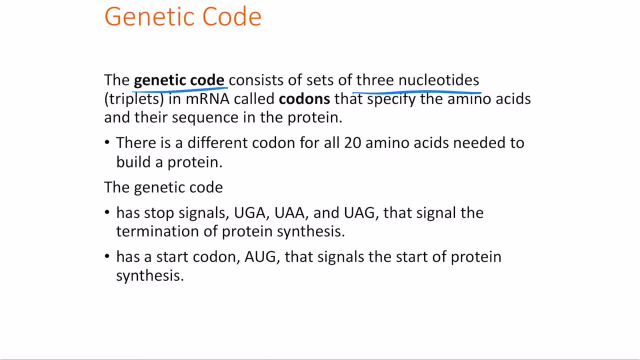 So the genetic code here consists of three nucleotides or triplets. in the mRNA We call them codons. So these codons are the ones that specify the amino acids that are in the sequence amino acids and their sequence in the protein. 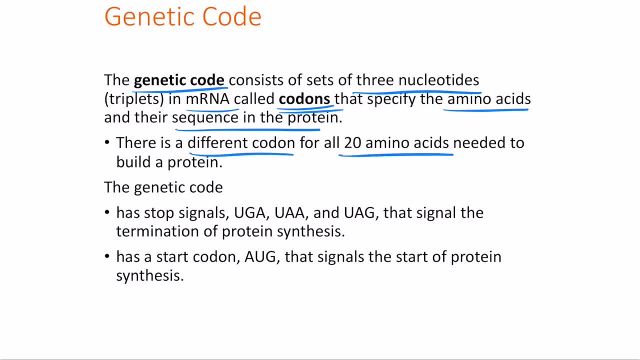 So there is a different codon for all of the 20 amino acids that are needed to build a protein. So the genetic code here has stop signals. So the stop signals are UGA, UAA, UAG. So that signals the termination of the protein synthesis. 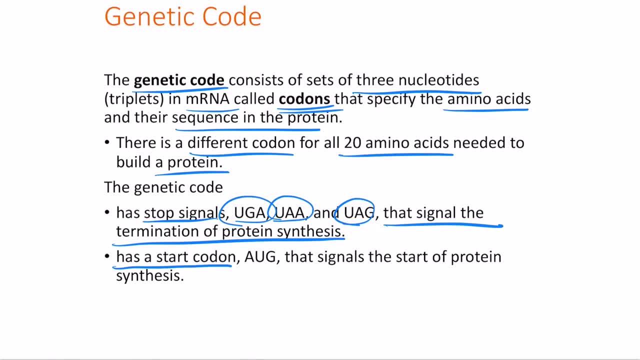 Now the genetic code has a start codon. The start codon is AUG. Remember that this is the start, starting codon. That signals the start of protein synthesis. So remember that all of the genetic message is not needed for the creation of the protein. 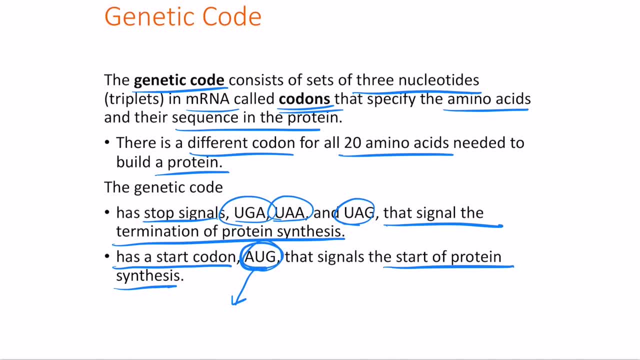 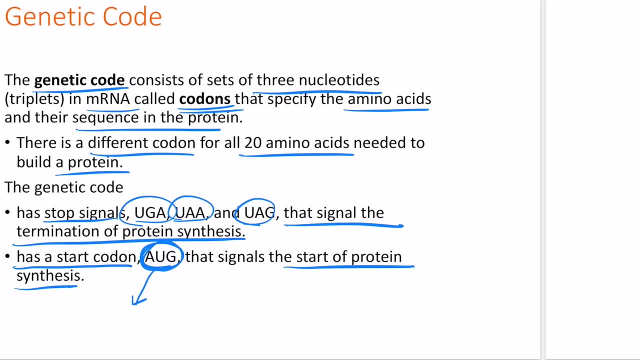 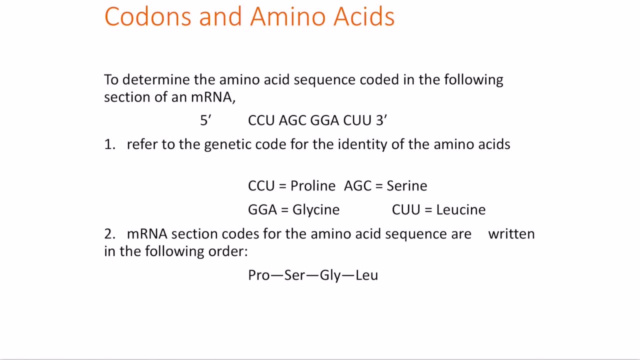 It only starts when it detects AUG formation. So the genetic code's AUG formation is the first part where the ribosome detects the creation of, starts the protein synthesis. So for example here to determine the amino acid sequence in the code, So we refer to the code here and we split each of the amino acids into three, three, three. 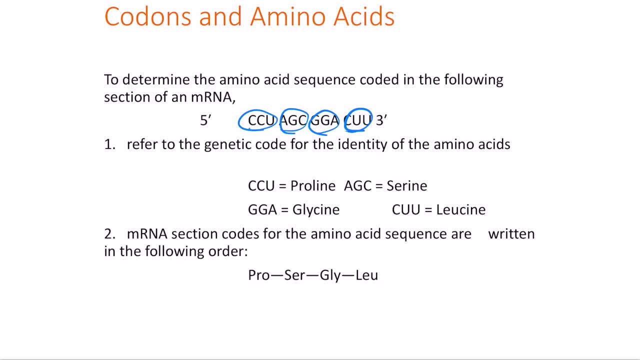 base pairs. So three pair, a pair of three, a group of three. So CCU here represents proline, AGC represents serine, GGA represents glycine and CUU represents leucine. So the final mRNA here is going to attach these, these of these structures, to create 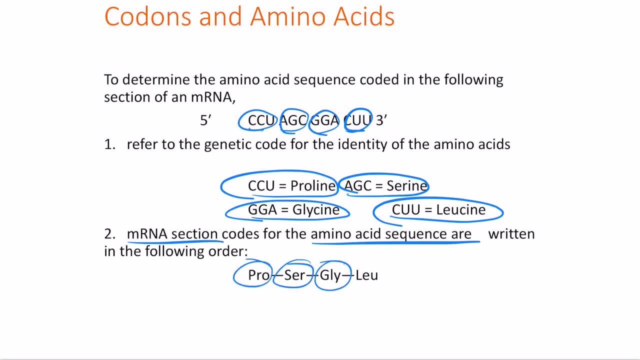 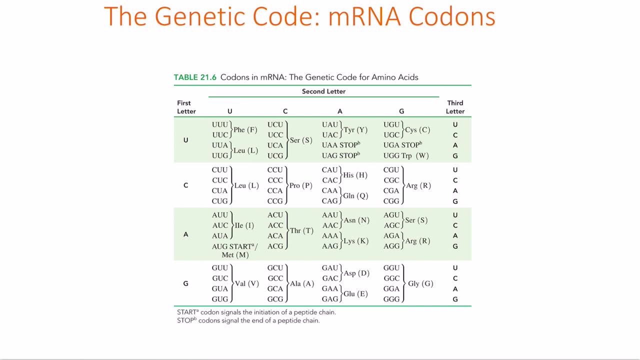 proline serine. so proline serine glycine leucine. So this is the polynucleotide that it generates from the mRNA sequence. Now what are the stop points where it can stop? So when you have UAA and UAG, it stops, UGA also it stops, but all of the following sequences: 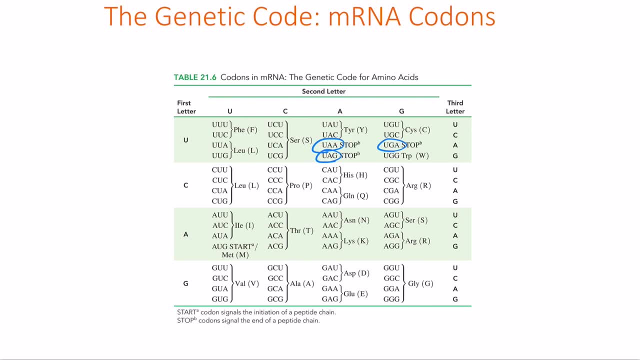 are representation of particular protein. here UUU and UUC can attach to create phenyl, phenyl aniline. You have GGU, GGC, GGA, GGG create glycine. So the third letter here, the first letter and the third letter are the ones that can. 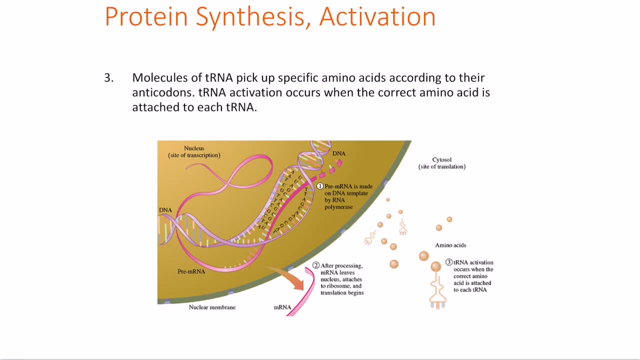 decide what type of structure it creates. So now, the molecules of the tRNA. what are the? what is the tRNA? tRNA is the transfer RNA are the ones that pick specific amino acids to according to their anticodons. 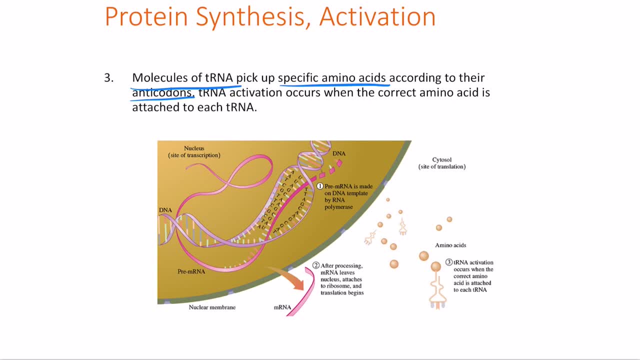 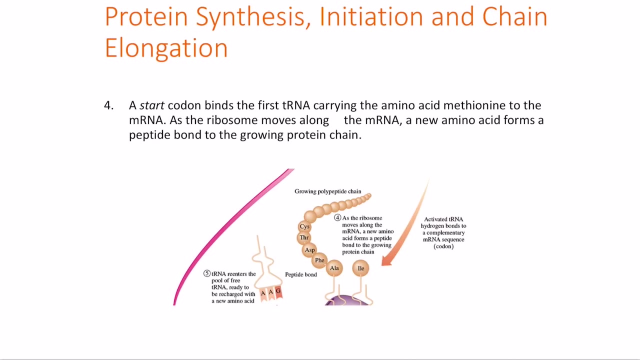 Remember that the codons are the ones on the RNA that are detected by the anticodons. The anticodons are the ones that are going to ask the tRNA to bring these specific amino acids that are needed to bond. Now the tRNA activation will occur when the correct amino acid is attached to the tRNA. 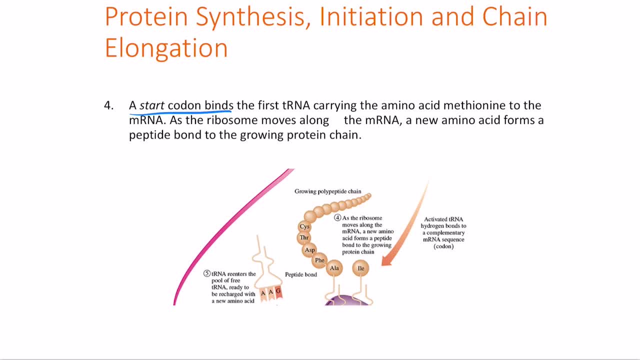 Now you have the RNA and tRNA. So a start. codon binds the first tRNA carrying the amino acid methionine to the mRNA. As the ribosome moves along the mRNA here, a new amino acid forms a peptide bond to the. 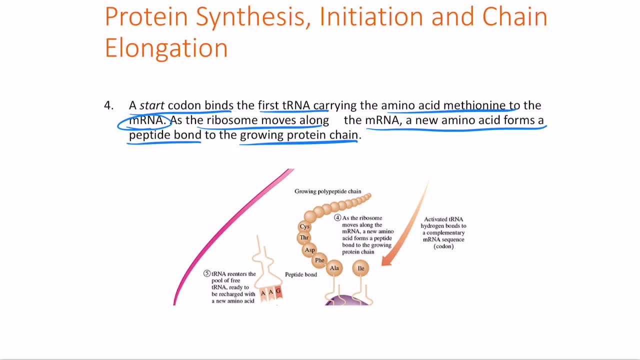 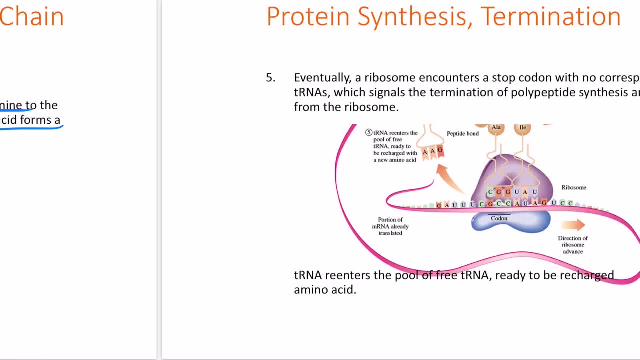 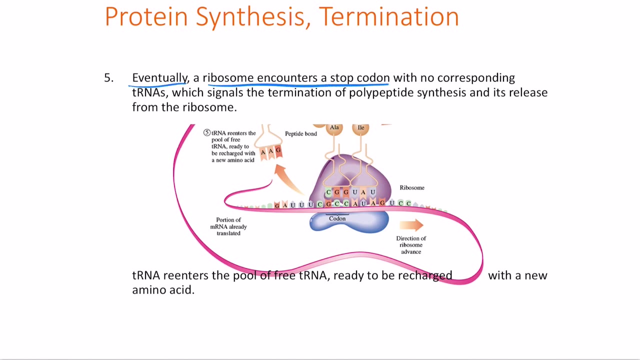 growing protein chain. So this is the fifth step. So first the structure. here Anticodon attaches itself, it bonds with the structure and then finally moves it along. So this way it creates the primary structure of the protein. So eventually a ribosome encounters the stop codon, when no corresponding tRNAs which signal. 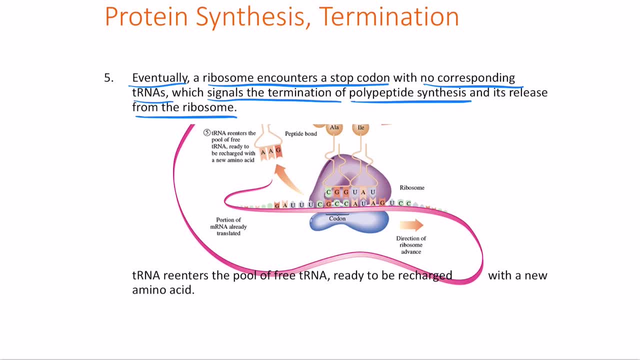 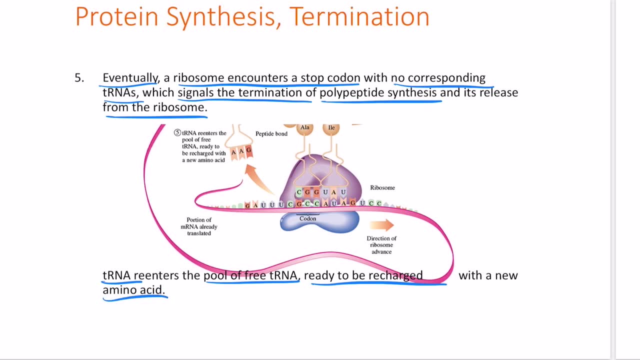 the termination of the polypeptide synthesis and it release from the ribosome. Then the tRNA re-enters the pool of free tRNA, ready to be recharged with a new amino acid. So this is the idea of translation inside the new amino acid. 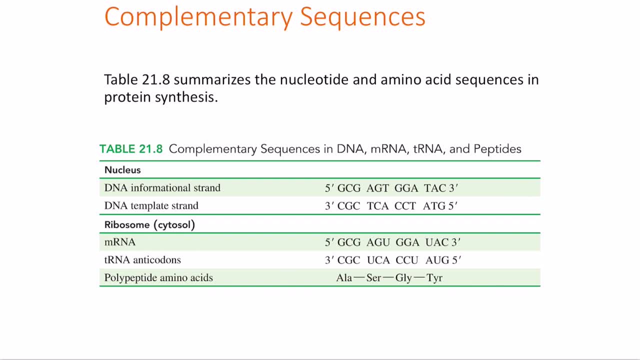 So, to summarize this, you have the DNA informational strand, you have the DNA template strand inside the nucleus. that generally ends up creating the mRNA. The mRNA then creates the tRNA strand, which is going to complement itself, and finally, the polypeptide amino acids are generally, finally, the ones that are created by the ribosome. 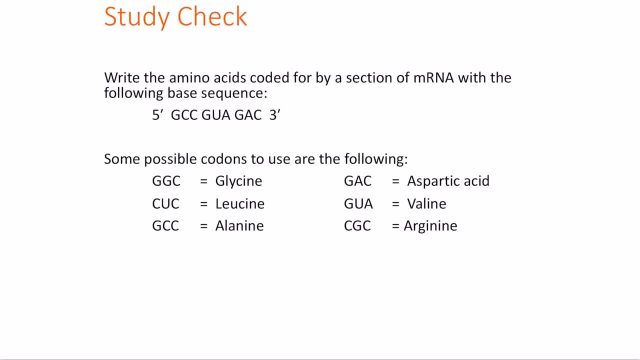 So one by one, by mixing it with x, such that that you Krishna SQL Sub blast. Alright, Now let us start a test based. If you can do that, celebrity people can let us know ESTP It is or is delete. then let us do that right. It is a little bit bougie. So the protocol for editing of a tRNA is like this: A and B. The protocol for making an A would be like this: So then A and B has to be computed here and the화를 is enough to predict O joint albumin. C and Q. Let us see if it fits here. Let's do a little bit over G somewhere. it is OK for me. Let me hold it one last time, my Thank So inter guitar. Thanks everyone, And thank you again. 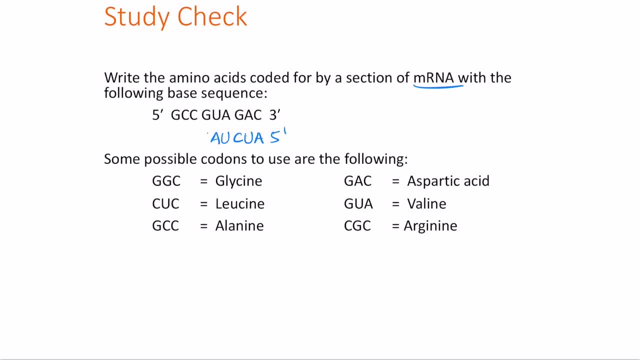 u, a, c, g, g, u and you have three pi, so it starts when it notices a, u, g, so when the sequence starts. so notice that here. i am sorry, they have already given us the mrna sequence, i'm sorry, so this is the sequence they have given us. so where would they? where? 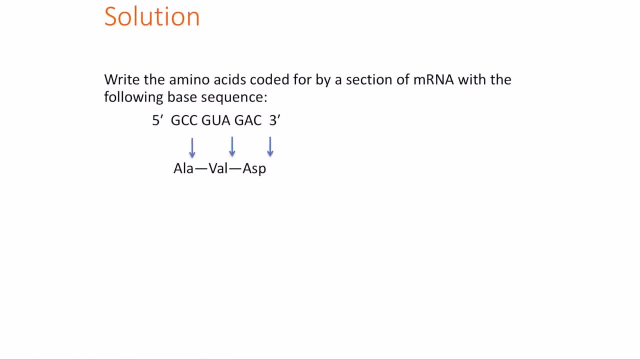 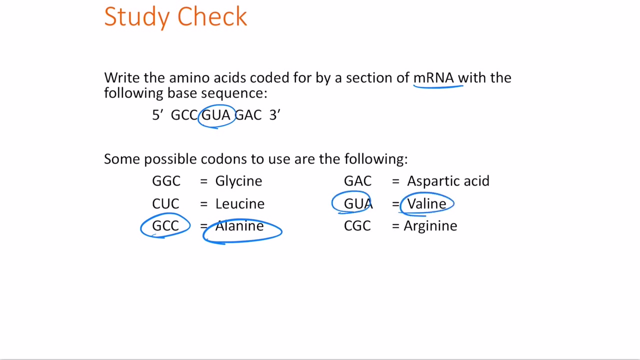 would you start now? so first you have the five prime. so the five prime and three prime are already in the structure. always read from five prime to three prime. so gcc here represents alanine, gua here represents valine and gac here represents aspartic. 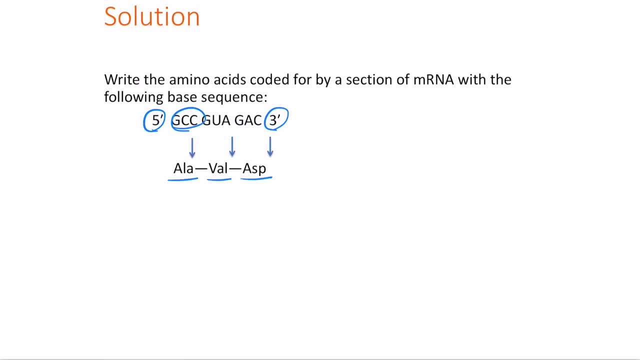 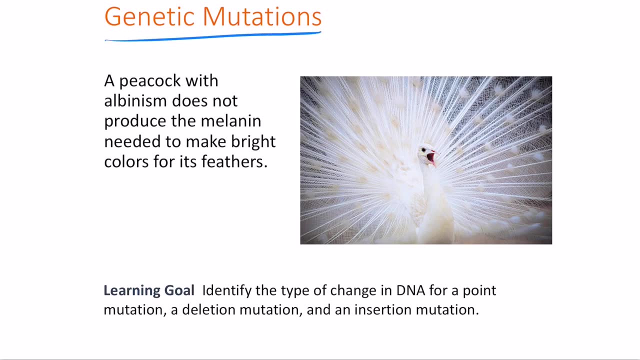 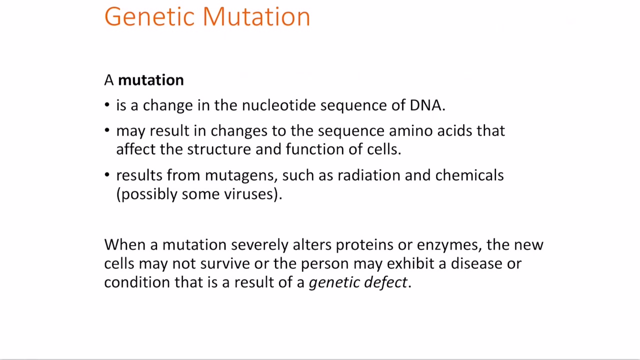 acid. so you end up with alanine, valine, aspartic acid. next let's talk about genetic mutations. so a common example of this is a peacock with albinism, so it does not produce the melatonin needed for its to make its bright colors, for its feathers. so mutation here is basically a change. 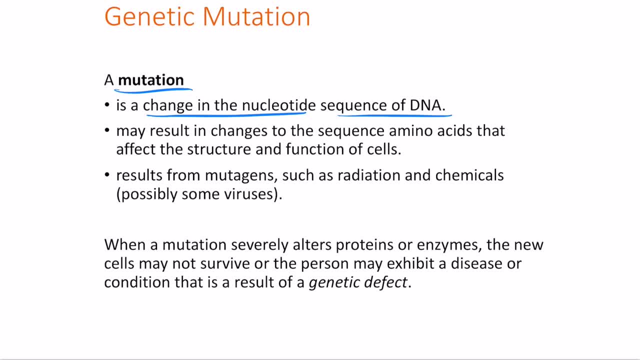 in the nucleotide sequence of the dna and it may end up resulting in the change of the sequence of amino acids that affect the structure and function of the cells. so these are generally from mutagens such as radiation and chemicals, possibly some viruses as well. so when a mutation 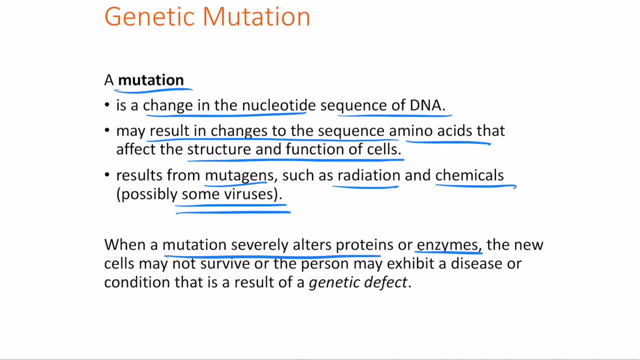 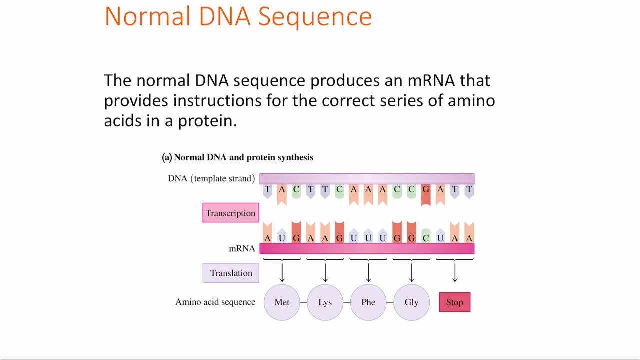 severely alters the proteins or enzymes, the new cells may not survive for long or the person may exhibit a disease. we call this a genetic effect. now the normal dna sequence produces the mrna that provides instructions for the correct series of amino acids in the protein. now if there is a kink in any of these processes, that ends up resulting 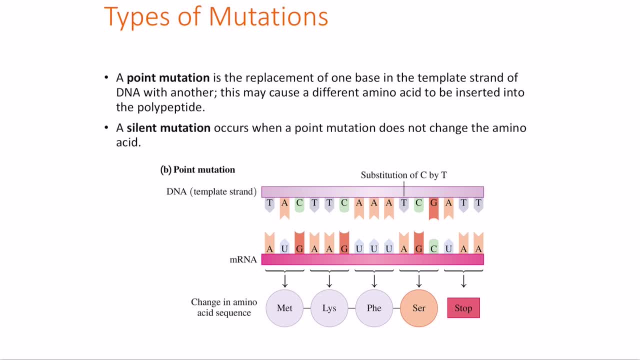 in the formation of the mutation. so a point mutation is the replacement of one base in the template strand of the dna with another. this may cause different amino acid sequence to be inserted into the polypeptide. now there is two. the other type of mutation is a silent mutation, where 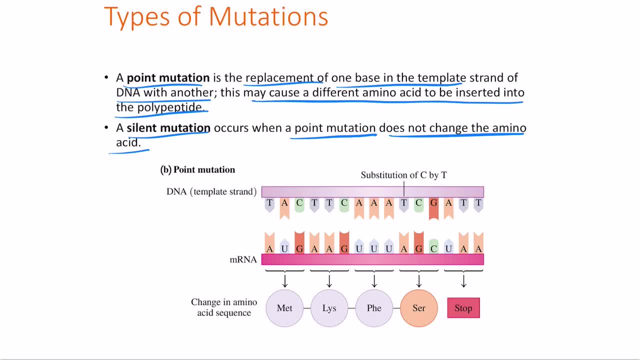 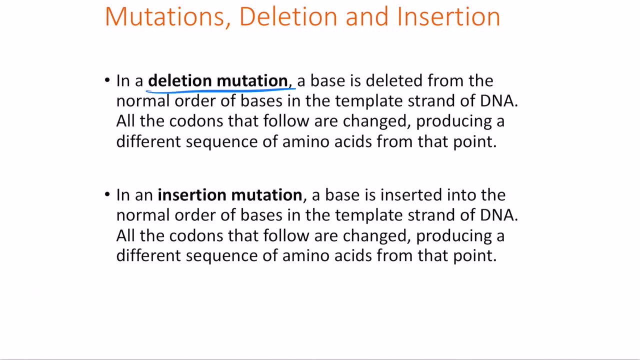 and when a point mutation does not change the amino acid sequence. so a point mutation will change the alter the amino acid sequence because it changes the dna, it changes the mrna and ends up changing the amino acid sequence. the next one is the deletion mutation, so where a base is deleted, 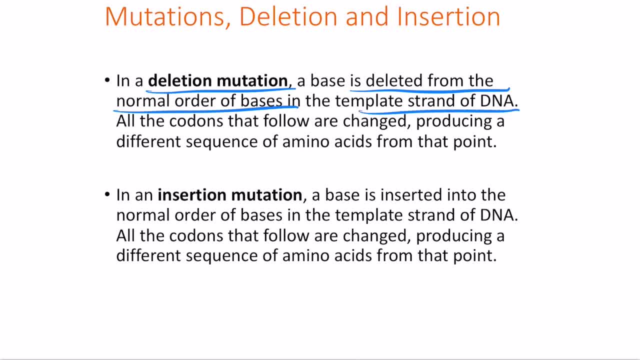 deleted from the normal order of bases in the template strand of the DNA, and all the codons here are following, or changed, producing a different sequence of amino acids. from that point There is another one, called insertion mutation, where a base is inserted into the normal order of bases in the template strand of the DNA, and here all the codons that follow: 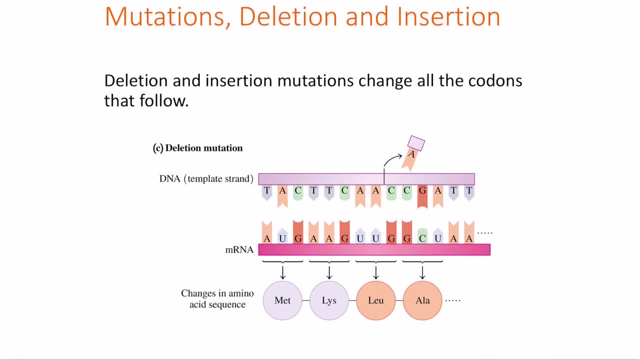 are changed, producing a different sequence of amino acid from that point. So this is an example of deletion mutation where one of the amino acid is one of the base pairs is gone, so one of the bases is gone, then it results in the formation of a different change. 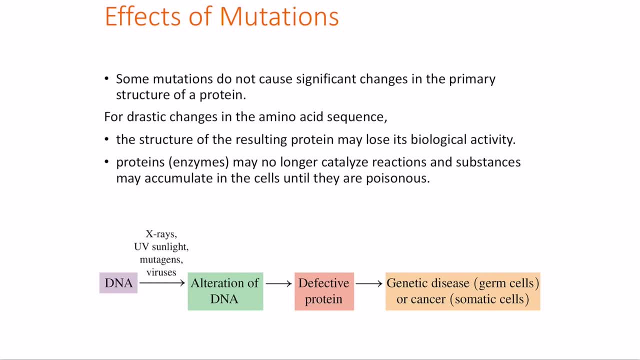 change the mutation of the amino acid chain. so what are the effects of mutation? so some mutations do not cause significant changes in the primary structure of the protein. so for diastric structures in the amino acid sequence the structure of the resulting protein may lose its biological activity. 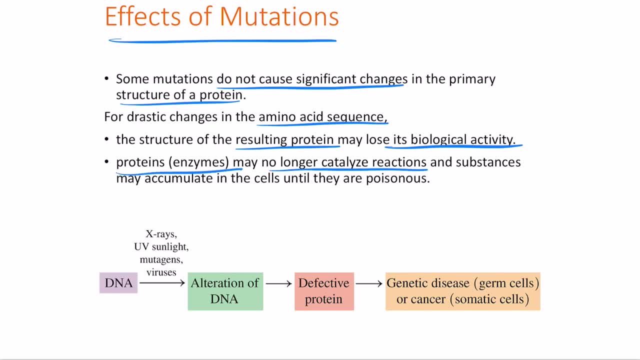 the proteins or the enzymes may no longer catalyze the reactions and substances may accumulate in the cell until they are poisonous. so, for example, dna undergoes a mutation, either by x-rays, uv light, mutagens or viruses, and that alters the dna. the altered dna can create defective proteins. the 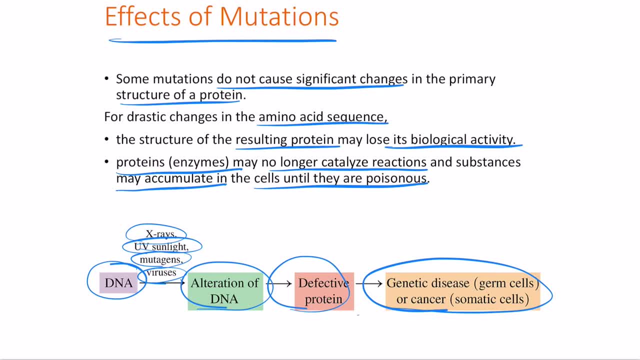 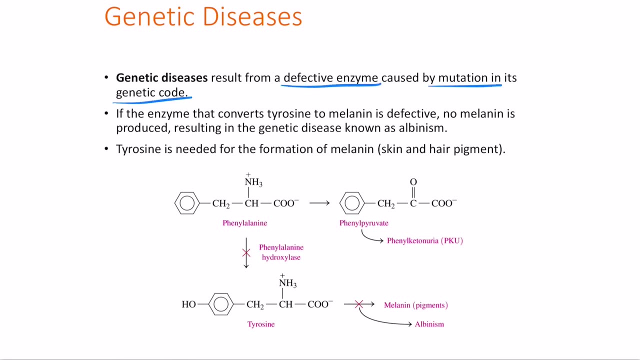 defective proteins, then can cause genetic diseases or cancer. so genetic diseases are generally formed due to germ cell mutation. cancers are generally caused due to somatic cell mutation, so genetic diseases result in a defective enzyme caused by mutation in the genetic code. you. if the enzyme that converts tyrosine to melanin is defective, no melanin is produced, and this here. 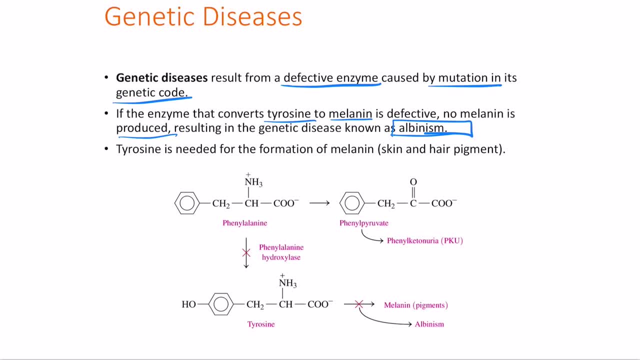 is called as albinism, which results in the formation of a white hair, no color, no skin pigments at all. so the tyrosine here is needed for the formation of melatonin. if there is no tyrosine formation, this ends up hurting the creation of melanin itself. so remember that. 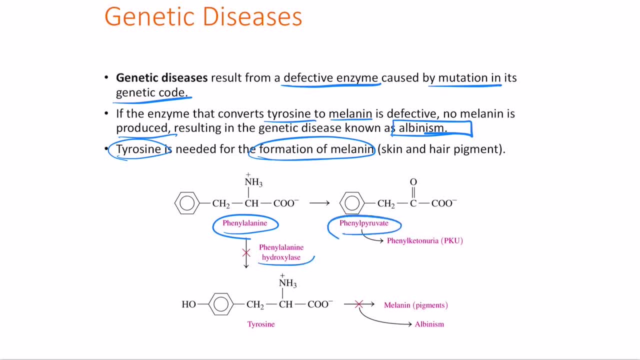 if there is no phenylalanine to phenylpyruvate. so if there is no phenyl phenylalanine hydroxylase, there is no tyrosine. if there is no tyrosine, there is no melanin. so this is this is what 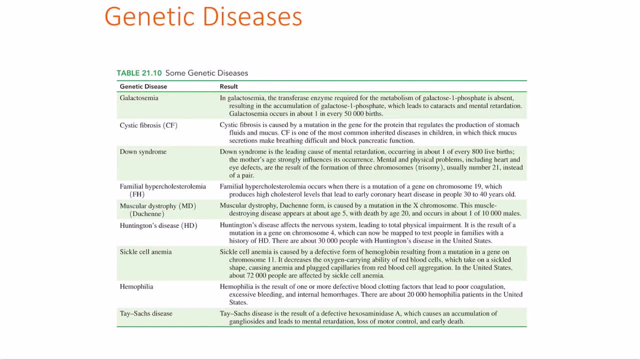 results in the formation of albinism. so these are some examples of different genetic diseases, some ranging from really small to really terrifying diseases. for example, galactosemia is the transferase enzyme required for the metabolism of galactose 1 phosphate, so it results in the accumulation of galactose 1 phosphate, which leads to cataracts and 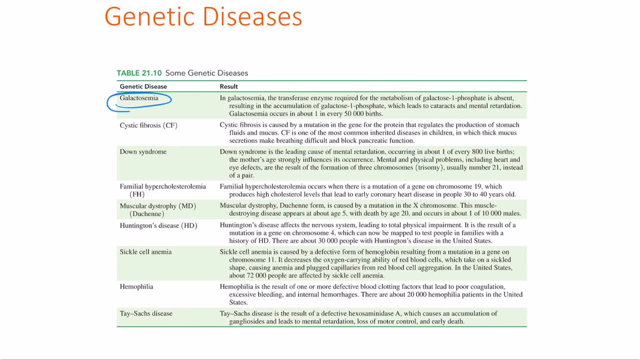 mental retardation. so it happens in about one of every 50,000 births. you have cystic fibrosis, which is a mutation in the gene of the protein that regulates the production of stomach fluid and mucus, so it is one of the most common inherited 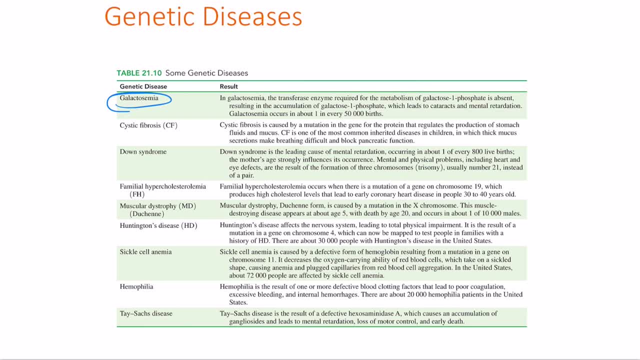 diseases in children where you can get a thick mucus secretion, making the difficulty in breathing and can create, can block the pancreatic function. you have down syndrome, which is the leading cause of mental retardation, which occurs in about one of every 800 live births. so the 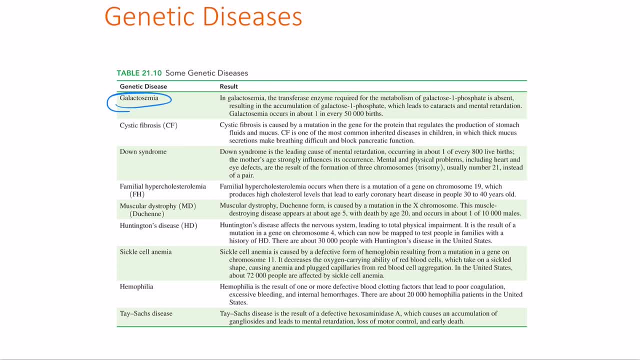 mother's age generally strongly influences its occurrence. so the mental and physical problems, including heart and eye defects, are the cause of the malignant and the intestinal. the result of these three chromosomes- and usually number 21- is the one- that, instead of a pain, you have familial hypercholesterolemia, which occurs when you have a mutation in the gene. 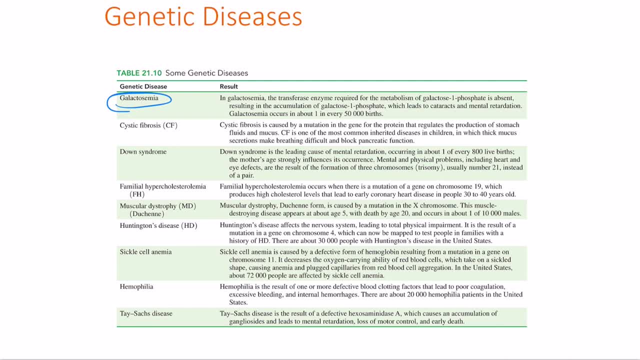 on the chromosome 19, which results in high cholesterol levels that can lead to early coronary heart diseases in people with 30 to 40 year olds. you have muscular dyotropy, you have huntington disease, you have sickle cell anemia, you have hemophilia, you have t-sex syndrome- these 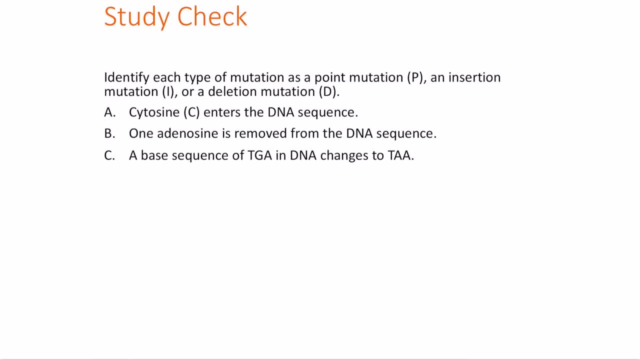 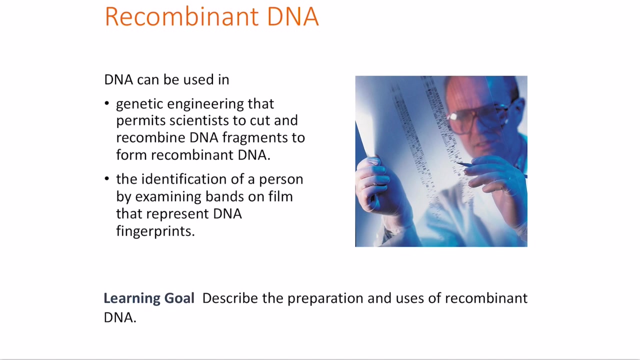 are all examples of genetic diseases. so pause the video right here and try to answer these questions. next let's talk about recombinant DNA. so DNA here can be used in genetic engineering, and that permits scientists to cut and recombine DNA fragments to form recombinant DNA, so the identification of a person's by examining the 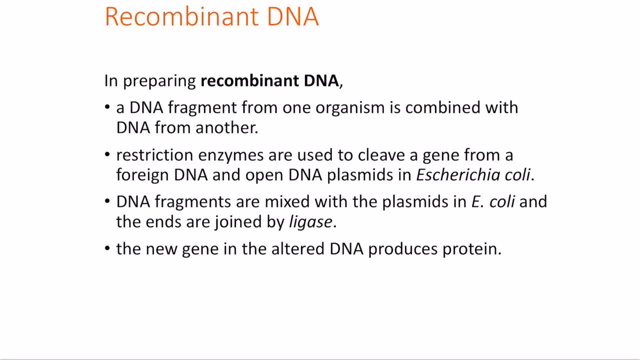 bands on a film that represents the fingerprints here. so the in process of, in preparing the recombinant DNA, we are taking a DNA fragment of one of one organism and then we combine it with DNA from another. so we have restriction enzymes that are used to cleave a gene cleave here. 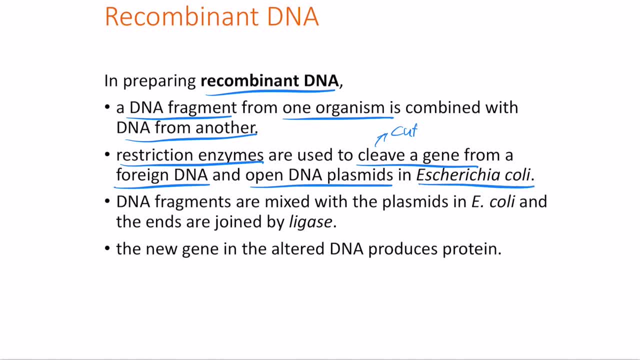 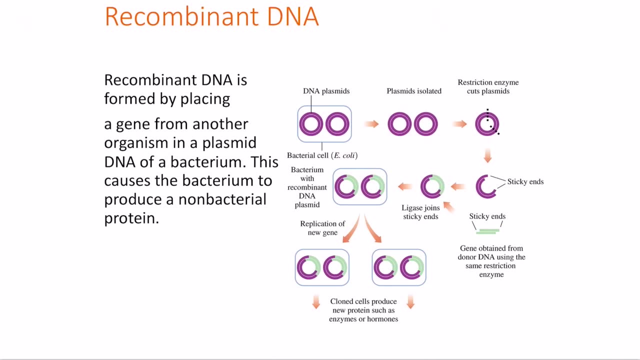 and open DNA plasmids in Escherichia coli or E coli. so the DNA fragments are then mixed with the plasmids in E coli and the ends are joined with ligase and the new gene is in the altered DNA produces a protein. that protein is what ends up creating the final answer that you need, so the 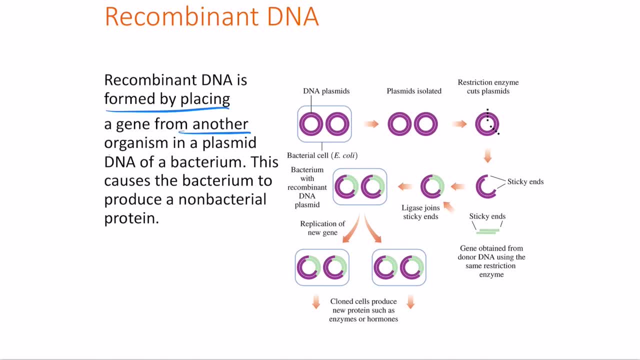 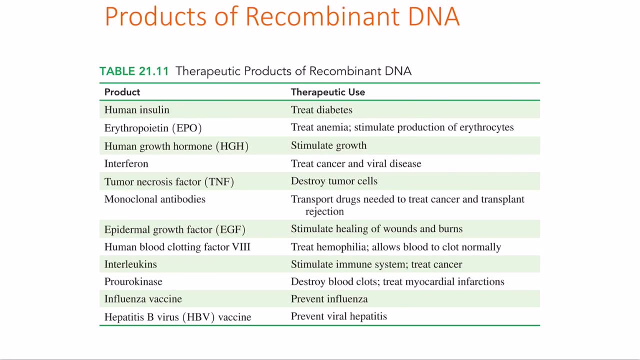 recombinant DNA is formed by placing a gene from another organism in the plasmid DNA of the bacterium, so this causes the bacterium to produce non bacterial DNA. so the non bacterial DNA is then the result of what are the that can be used from different products. so these are common. 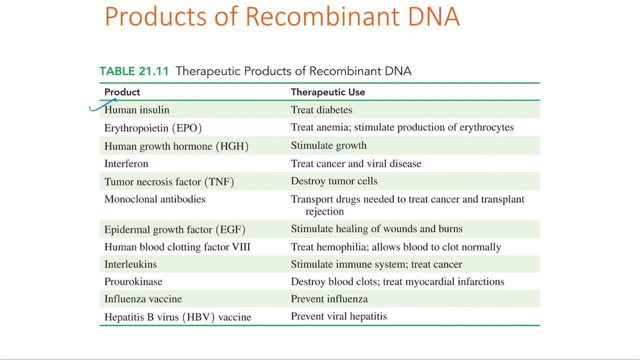 products that we have seen. first one is humor in insulin that is produced by the common in DNA. you have erythropoietin, which is used to treat anemia and stimulate production of erythrocytes. you have human growth hormone, which is used to stimulate growth. you have interferon, which is used to treat 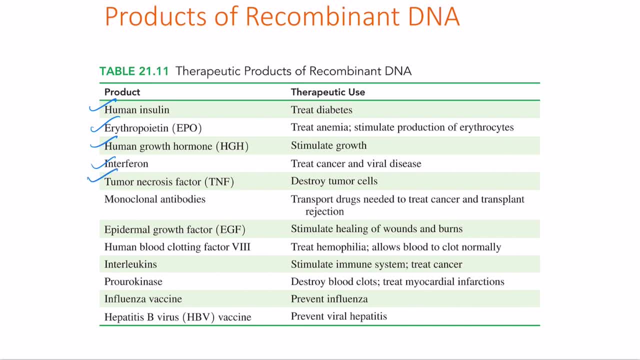 cancer and viral diseases. you have tumor necrosis factor, TNF, which is used to destroy tumor cells. you have monoclonal antibodies, which is one of the easiest ways to transport drugs needed to treat cancer, and transplant rejection, where we take antibodies from one person and try. 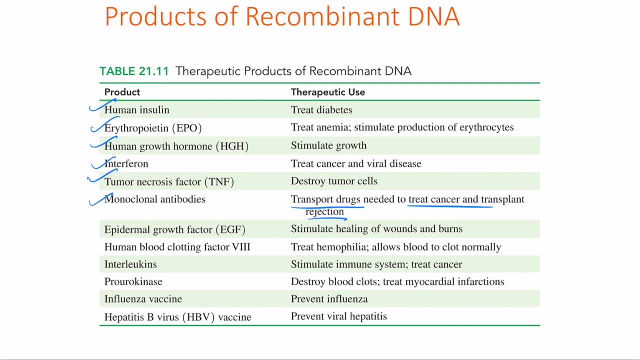 to create antibodies for other person. you have epidermal growth factors, which are used to stimulate healing of wounds and burns. you have human blood clotting factor 8, which is used to treat hemophilia and allows blood to clot normally. you have interleukins, which can stimulate immune. 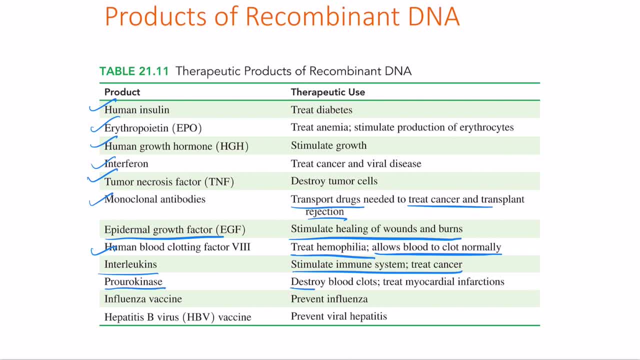 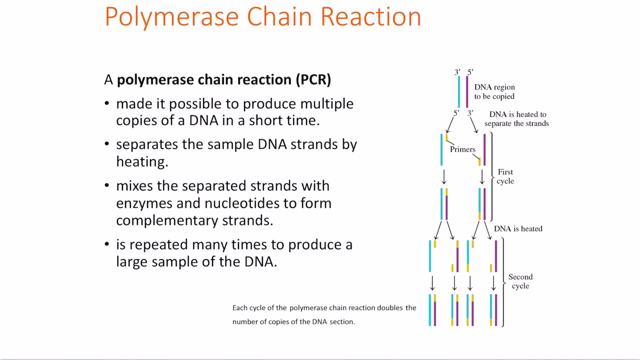 system and treat cancer. you have pure urokinase, which is used to destroy blood clots and treat myocardial infractions. you have influenza vaccine, which is also created by the common in DNA used to prevent influenza. you have hepatitis B vaccine, which is used to prevent viral hepatitis, and the next process that is used in the DNA process is PCR. 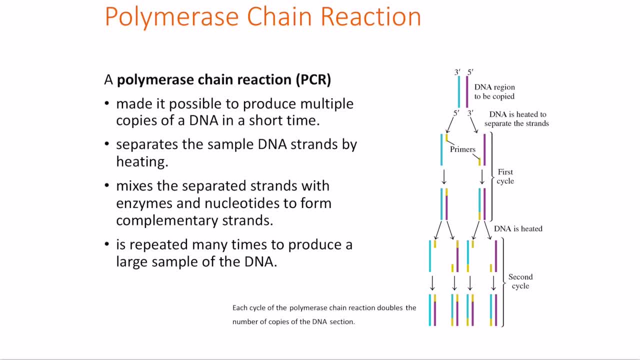 or polymerase chain reaction. so polymerase chain reaction involves making it so it makes it possible to produce multiple copies of a DNA in a short time. so it separates the sample DNA strands first and then mixes the separate strands of the with the enzymes and nucleotides to form 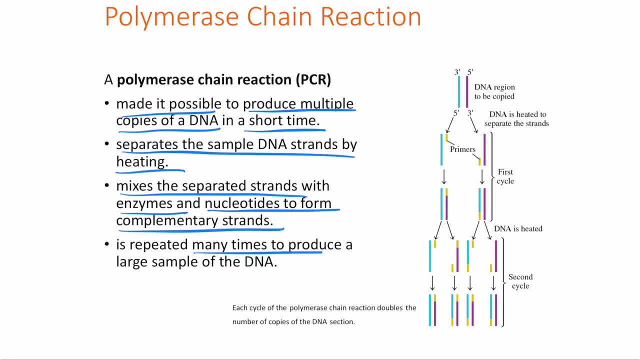 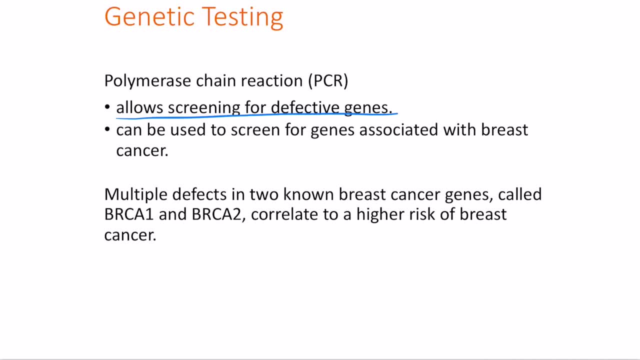 complementary strands and if you repeat the process enough times it can create a large sample of the DNA and the polymerase chain reaction allows screening for defective enzymes. it can be used to screen for genes associated with breast cancer. so multiple defects in two known breast cancer genes are called BRCA1 and BRCA2 are generally used to correlate to a high 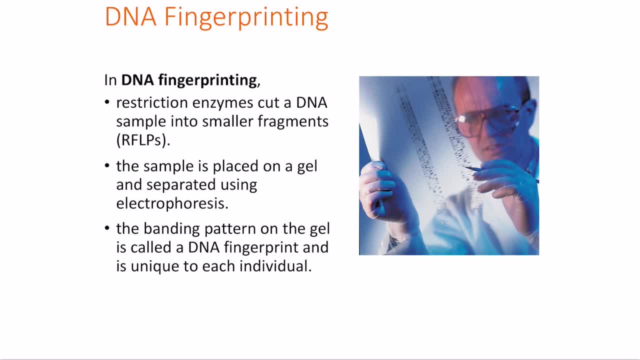 risk of breast cancer. next process is DNA fingerprinting. so DNA fingerprinting is used in the restriction enzymes to cut a DNA sample into smaller fragments, and then the sample is placed on a gel and separated using electrophoresis. the banding pattern on the gel is called as a DNA fingerprint and it 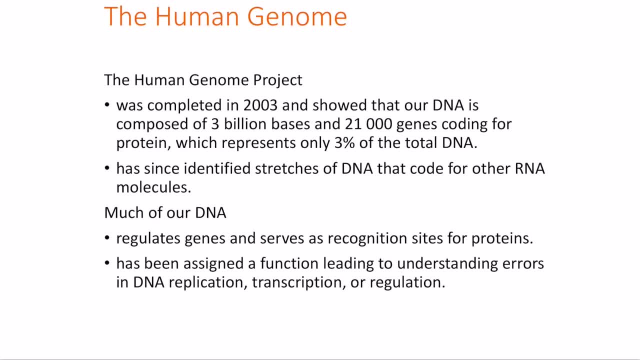 is unique to each individual, so the next one was the human genome. the human genome project was the first project that was completed in 2003, and it showed that our DNA is composed of our 3 billion and 21,000 genes coding for the protein, which represents only about three percent of the total. 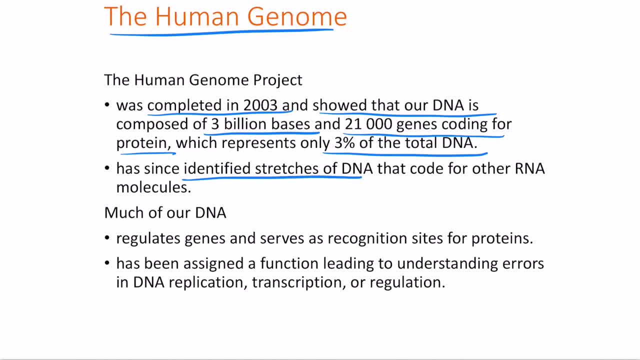 DNA, and it has since identified stretches of the DNA that code for other RNA molecules. so so much of our DNA is used to regulate the genes and serve as recognition sites for proteins, and it has been assigned a function leading to understanding errors in DNA replication. transcription of. 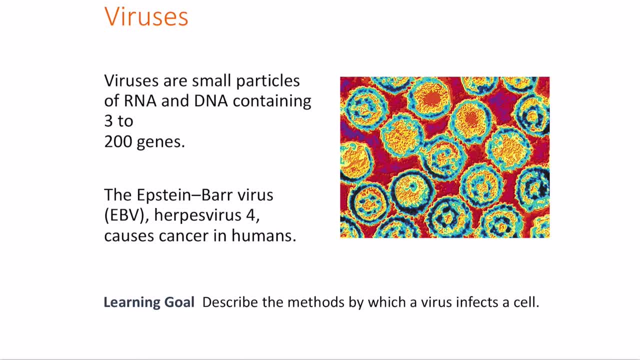 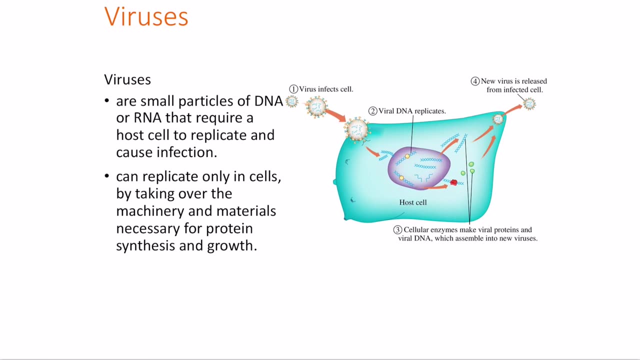 regulation. and the last step is viruses. so viruses are small particles of RNA and DNA containing up to three to 200 genes. examples of these are the Epstein-Barr virus, herpes virus that can cause in humans. so viruses are really small particles of DNA or RNA. we classify them into two. 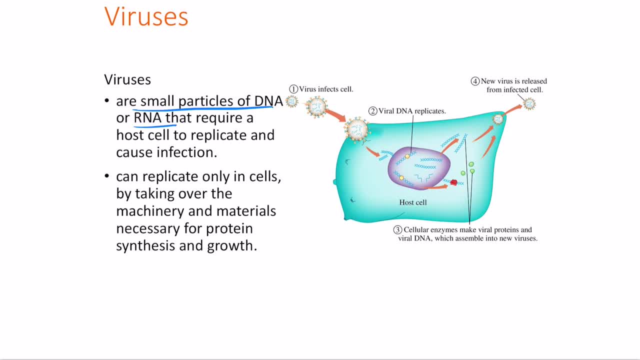 types of viruses, whether one is a DNA virus, the other is an RNA virus, so that require host cell to replicate. the cell function to replicate and cause infection. so replication involves creation of new molecules. so when a virus infects a cell it transfers the genetic material into. 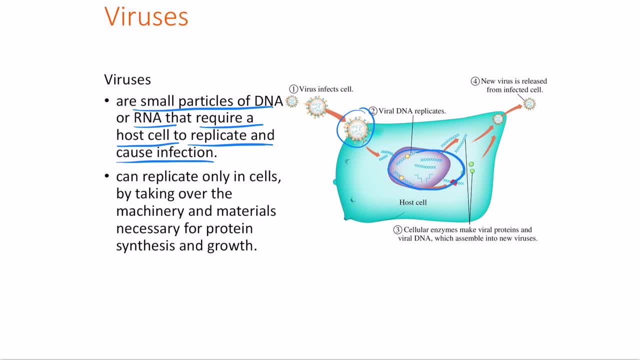 the cell and uses the cell as a factory and then ends up creating more and more new viruses and it generally uses up the cell to make sure that uses up the entire energy of the cell and finally kills the cell and the newly formed viruses then in fact then attack the new cells. then 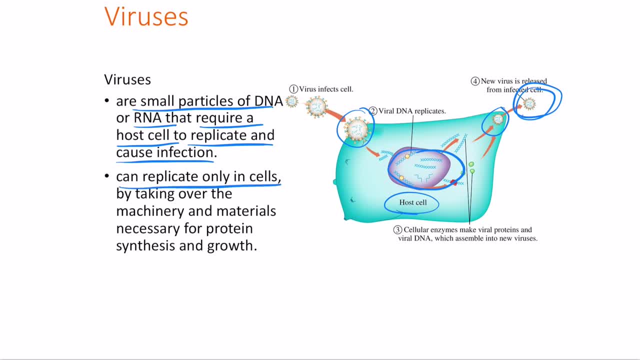 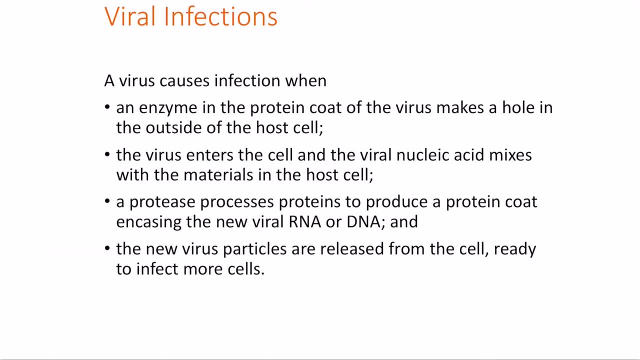 finally creating more and more viruses so they can replicate only in cells by taking over the machinery and materials necessary for protein synthesis and growth. so a virus infection, virus causes infection. when you have an enzyme in the protein port of the virus that makes a hole in the outside of the host cell, the virus enters the cell and the viral 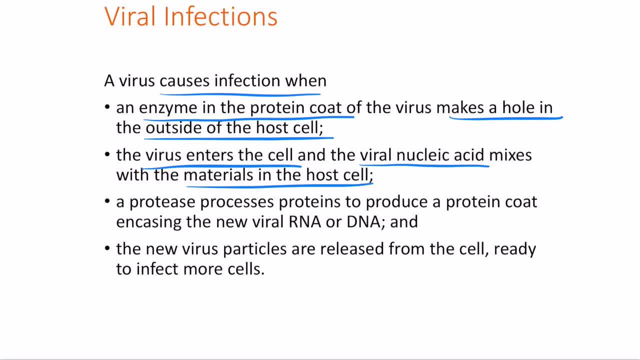 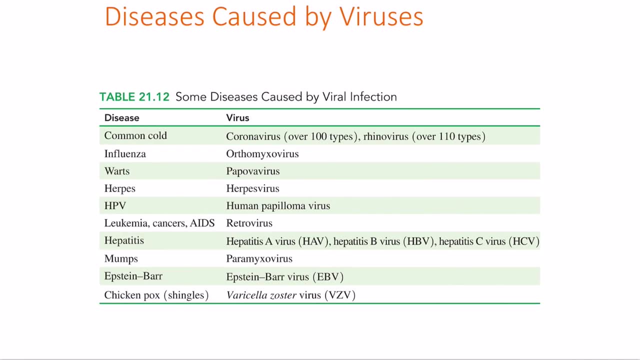 nucleic acid mixes with the materials in the host cell, a protease processes processes the proteins to produce a protein court encasing of the new viral RNA or DNA. then the new virus particles are released from the cell and then ready to infect more cells. so common viruses. you have common cold. 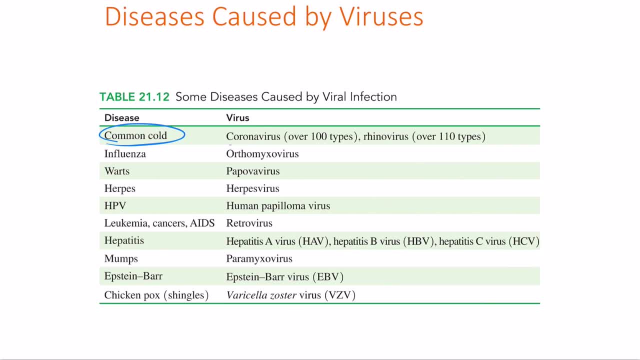 which is generally called by the over 100 types of viruses called as the coronaviruses, the, the corona word. corona comes from the idea that they look like crowns, so they have like the crowns on them and you have rhino viruses. there are about 110 types of them. you have influenza, which is 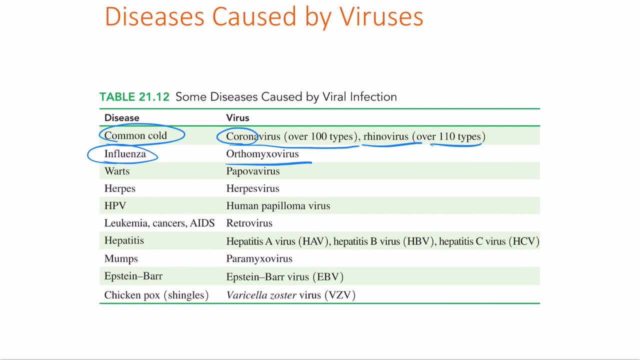 caused by ortho orthomyxovirus. you have warts that are caused by papo papovirus, herpes by herpes virus, HPV by human papillomavirus, leukemia, cancer and AIDS by retroviruses, hepatitis by hepatitis a, hepatitis B, hepatitis C viruses, mumps by paramyxovirus, Epstein-Barr virus, obviously. 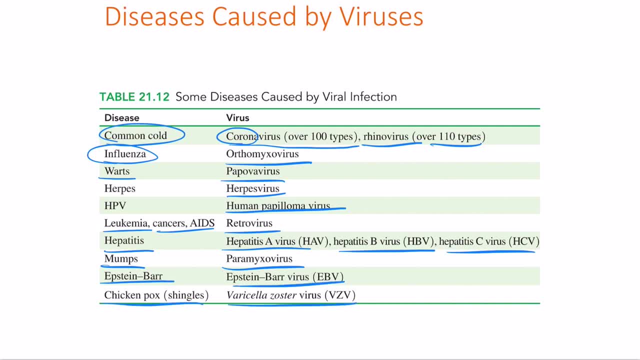 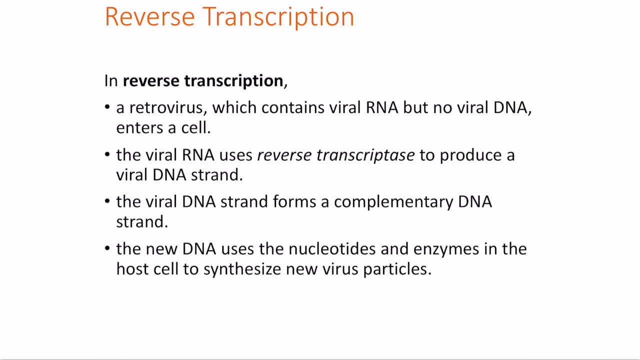 again: Epstein-Barr virus. chickenpox is caused by varicella zoster virus. so these are different viruses and the diseases that can they can cause. now there is a process called reverse transcription. that is important. so in reverse transcription, what is going to happen is that 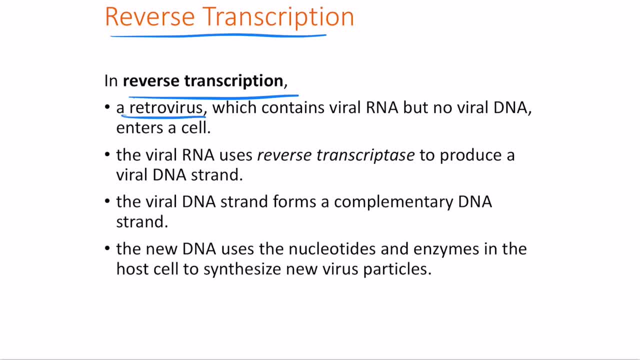 a retrovirus is an example of a virus that can create this process in your cell, where it takes the viral RNA. it generally does not contain any DNA, but only contains RNA. so but for it to undergo the transcription process, it needs the. it needs the DNA. so what it does is: 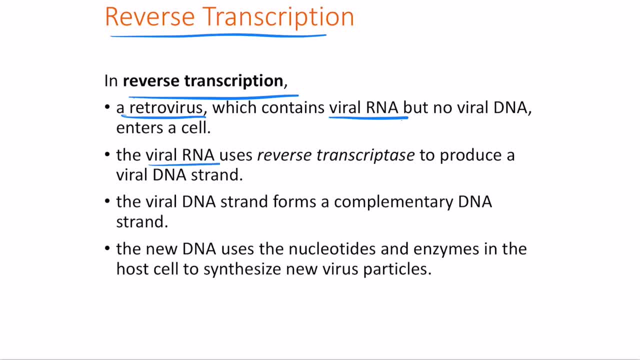 that to replicate itself. it basically takes the viral RNA here, uses reverse transcript trace to create a viral DNA strand. the viral DNA strand then creates the complementary DNA strand, finally ending up creating the new DNA using the nucleotides and the enzymes in the host cell to synthesize the new viral particles resulting. 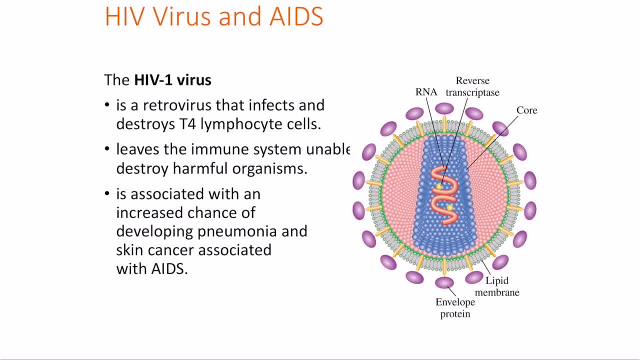 in the formation of new, new viruses. so one of those viruses is HIV virus. HIV virus is an example of a retrovirus, so it infects and destroys the t4 lymphocyte cells and it leaves the immune system unable to destroy the harmful organisms, because T cells themselves are the ones that that are. 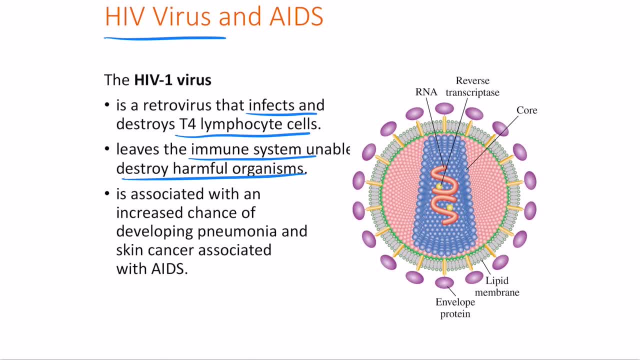 responsible for protecting your body, but if the T cells themselves are infected, then that is the where you are going to get the virus and you are going to get the virus, you are going to get the virus. you end up leaving the immune system to ruins, and it's generally associated with increased chance. 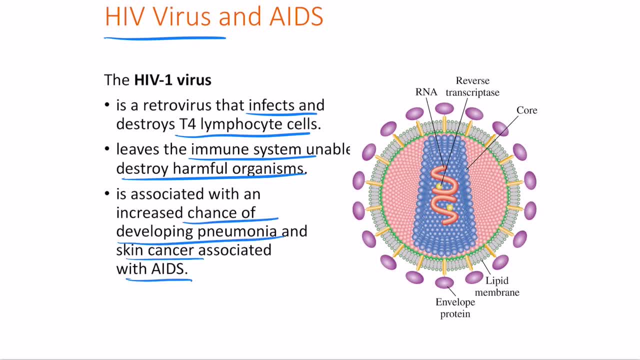 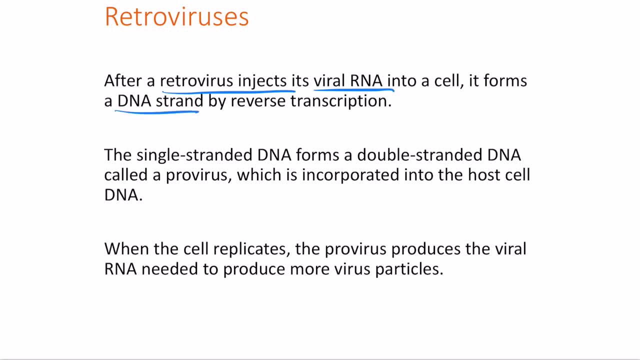 of developing a pneumonia skin cancer associated with AIDS. so retroviruses: after a retrovirus injects its viral RNA, it forms a DNA strand by viral reverse transcription. remember that DNA to RNA is called transcription, so the reverse transcription here is from RNA to DNA. so the single-stranded DNA then forms a double-stranded DNA. we call that a provirus. 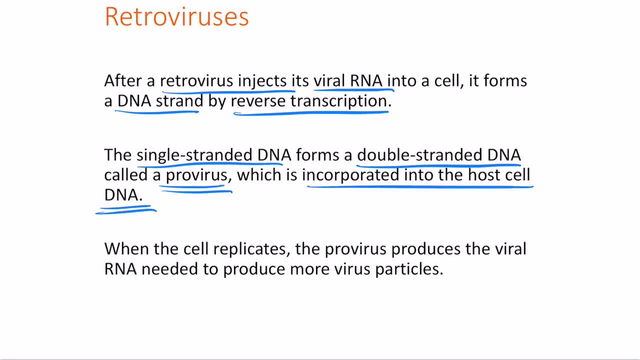 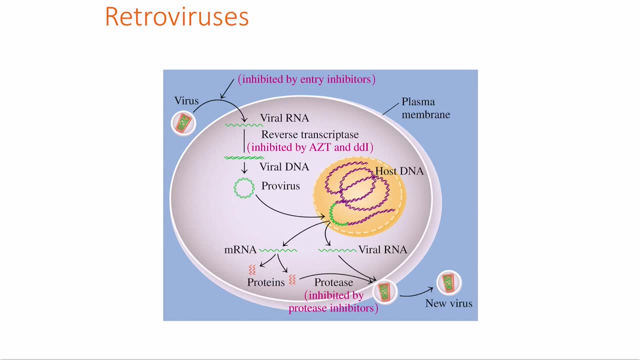 which is then incorporated into the host cell DNA, finally ending up creating the replication. so where the cell replicates, the provirus produces the viral RNA needed to produce more virus particles. so this is the function of a retrovirus. so one of those is inhibited by protease inhibitors. so 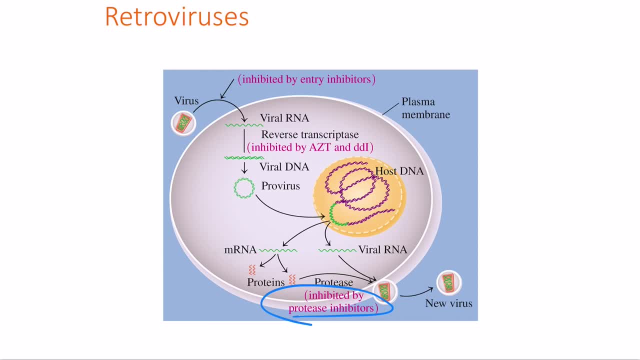 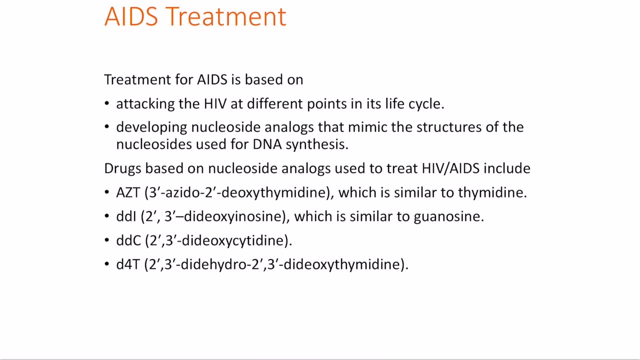 protease enzyme is the one that inhibits one of these processes. if the if they are overcome, then that is where you end up creating the reverse transcription processes. so one of the things that is being used in the AIDS treatment here is based on attacking the HIV at different points in its 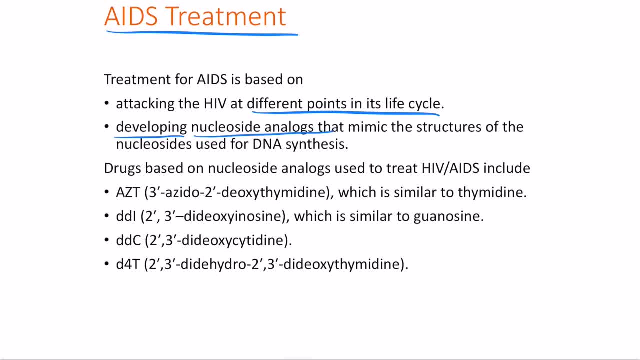 life cycle. first is to developing the nucleoside analogs that mimic the structures of the nucleosides used for DNA synthesis, and then drugs that are based on nucleoside analogs, to include AZT, DDL, DDC and D40, so which are similar to the original ones that are present on the virus. so we use 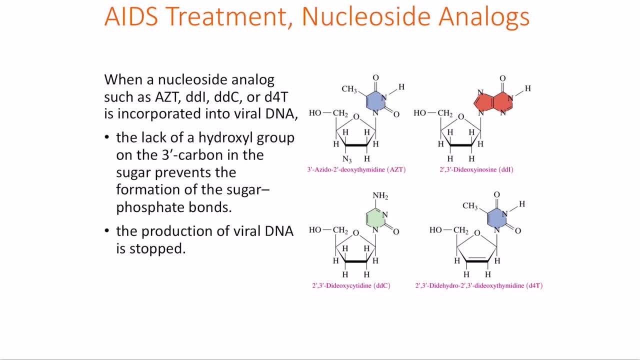 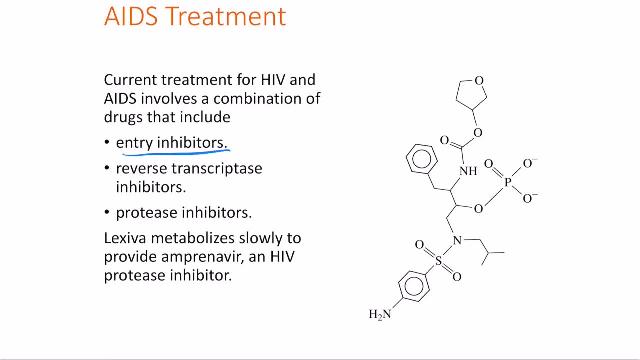 nucleoside analogs that stops the viral DNA from undergoing reverse transcription and to stop the reverse transcription process. so they can be done by using entry inhibitors. where you can stop the entry of the virus, you can use reverse transcription inhibitors where you can stop the replication of the virus. you have protease inhibitors which can stop the new. 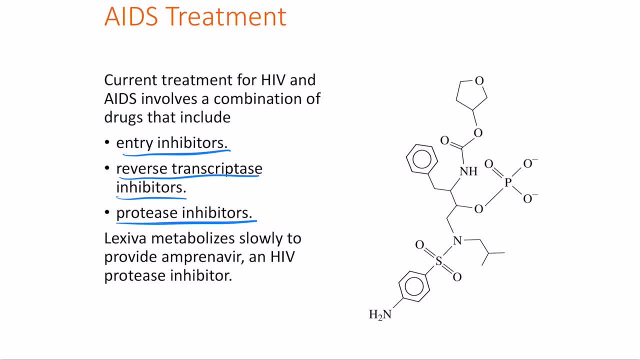 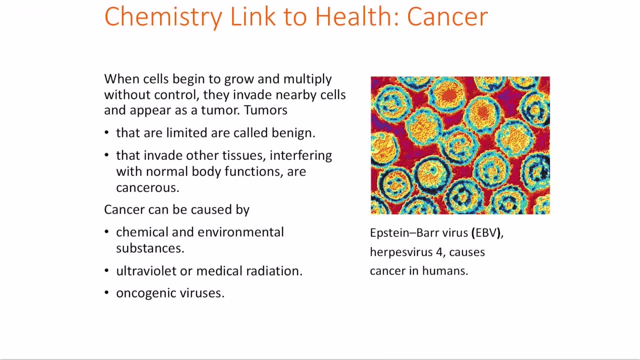 virus form to come out of the cell. so you have lexiva, which metabolizes slowly to provide amperin away. so which is the HIV protease inhibitor? next is the chemistry linked to health. let's start with cancer. so when cell begins to grow, they multiply without control and then invade the 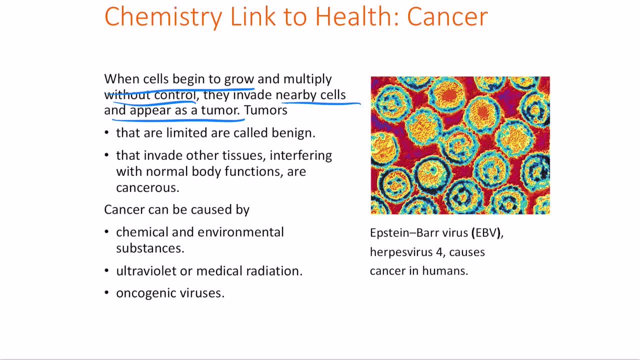 nearby cells and appear as a tumor. now the tumors here are limited to what we call. there are limited ones that are called benign, and there are ones that can invade other tissues, interfering with the normal body function. we call them cancerous ones. so these can be caused by chemical and 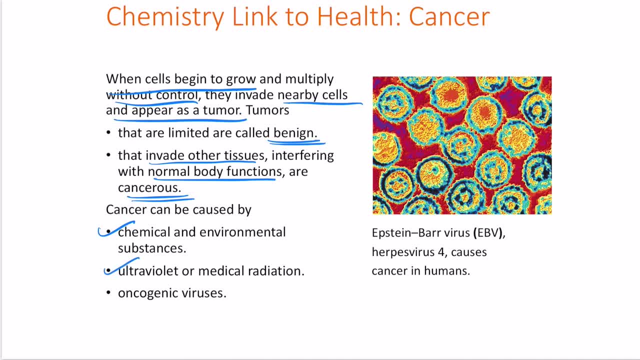 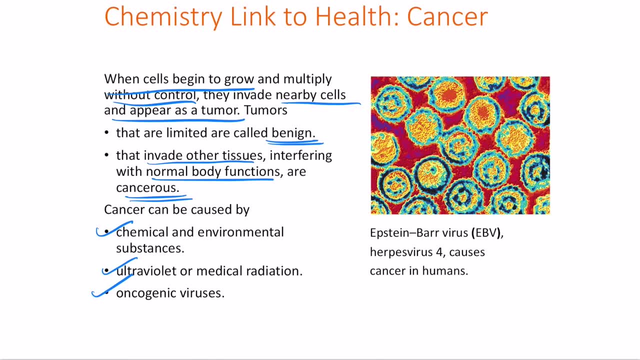 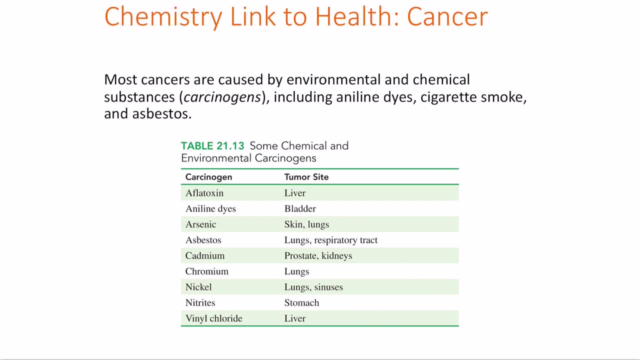 environmental factors, ultraviolet or medical radiation, oncogenic viruses. so, for example, Epstein virus is the one that can cause herpes 4 virus and Epstein-Barr virus can cause cancer in humans. so most of the cancers are generally caused by environmental and chemical substances. we call them carcinogens and include aniline dyes, cigarette smoking and asbestos. you have. 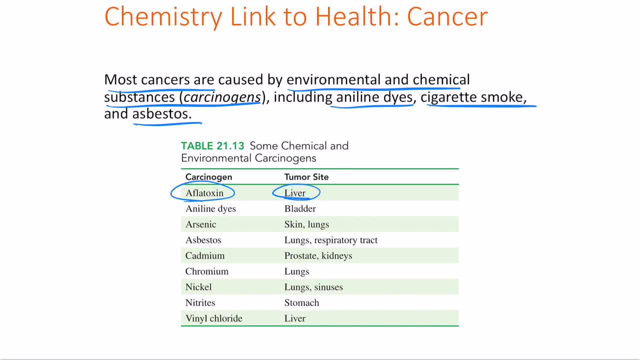 aflatoxin, which is the tumor site for liver. aniline dyes can create the bladder cancer. arsenic can cause skin and lung cancer. asbestos can cause lung and respiratory tract cancer. cadmium can cause prostate and kidney cancer. you have chromium that can cause lung cancer. nickel: 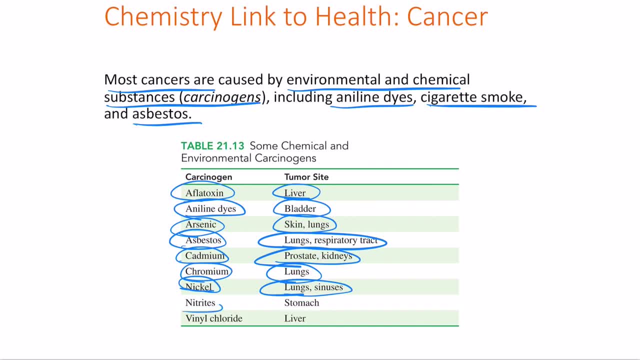 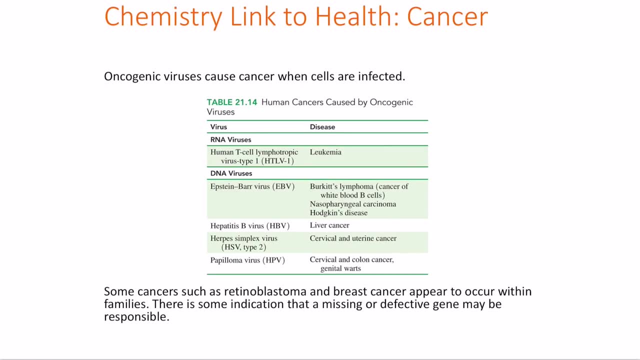 can cause lung and sinus cancer, nitrites can cause stomach cancer and vinyl chloride can cause liver cancer. these are what we call carcinogenic substances. you have oncogenic viruses that can cause the disease as well. for example, human T-cell lymph tropic virus type 1 or HTLV 1 can cause leukemia. DNA viruses such as Epstein-Barr virus can cause. 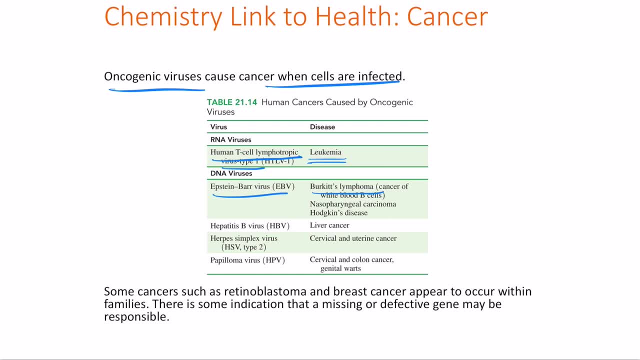 Burkitt's lymphoma, which is the cancer of the white blood B cells, and you can also cause nasopharyngeal carcinoma and Hodgkin's disease. you have hepatitis B virus, which can cause liver cancer. herpes simplex virus can cause cervical and uterine cancer. papillomavirus can cause cervical coron cancer and